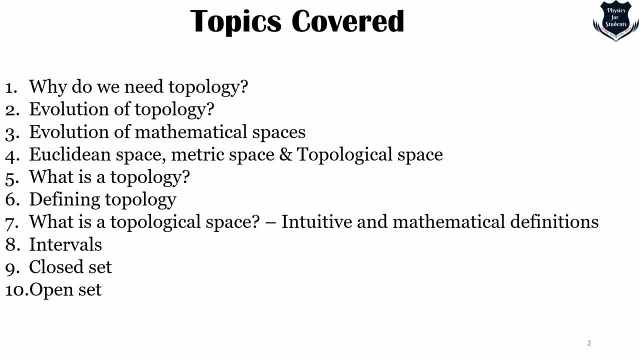 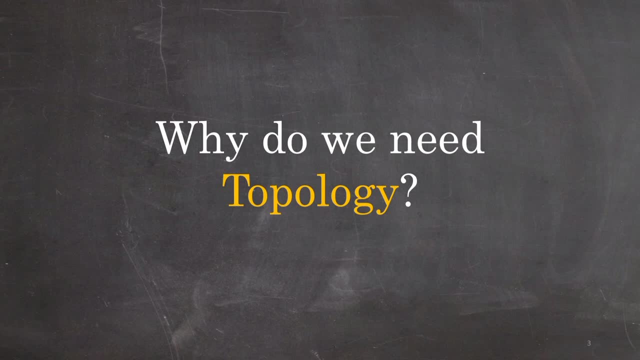 First of all, before going ahead, the most important thing that we need is that: why do we at all need the subject topology? I mean to say, if there is no topology, then what would have been the problem? If you look into the technological development of humans and 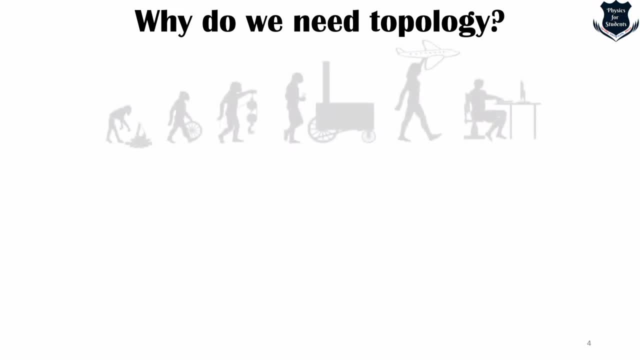 civilization or as a whole human race. you will always find that the technological development have taken place in order to make things easier. Each and every technology, starting from electronics to gadgets, to communication and everything these have been made in order to make things pretty easy, And topology is also not an exception. 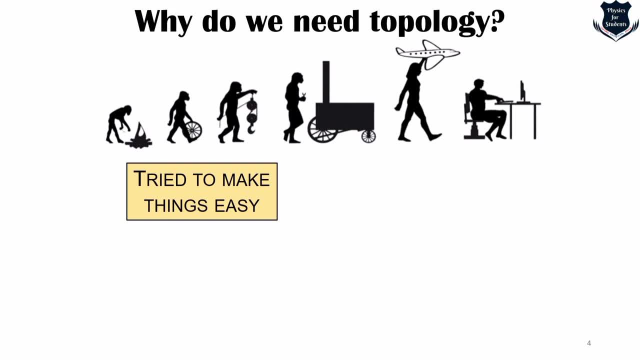 So if you look into these developments, the basic objective was to make and try to make things easy. Also, the gadgets which evolved slowly became smaller, which was earlier a little bit larger, And it also served on all purpose. It is not specific that it will. 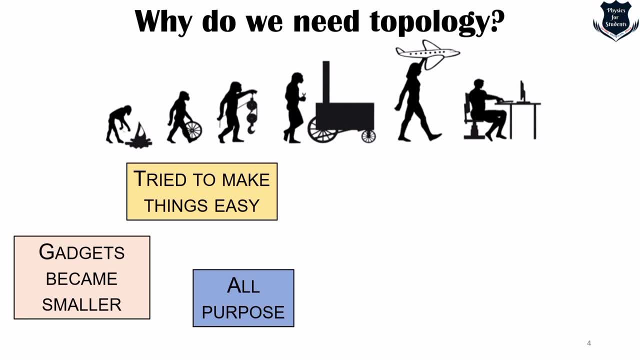 serve a specific purpose, like washing machine or communication, like talking over telephone, So it become an all purpose. Most importantly, it become easier to use and it become very user friendly. And, most important But last point, Is that we always- the human civilization, technological advancement- tried to make things. 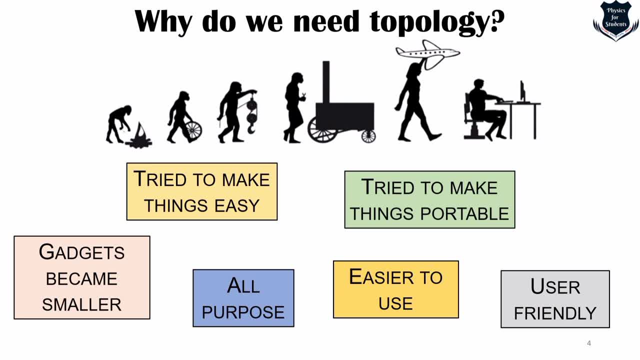 more portable. Now you might be wondering that am I teaching you history? No, But before going into topology, we need to understand that, because topology is also a human advancement, a thinking and a critical thinking advancement, which made mathematics much more easier. all purpose. 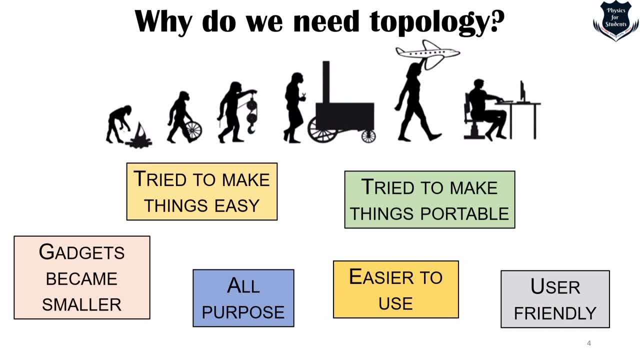 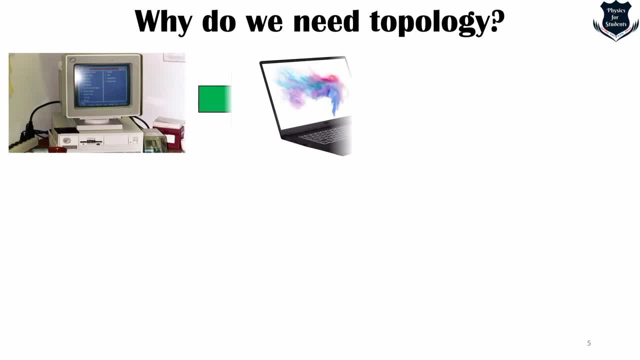 easier to use, user friendly and mathematics became more portable. So, as you see on your figure, this is an old cathode ray tube computer which was further generalized and became easy into a laptop. This I think you must have seen, or maybe somebody. 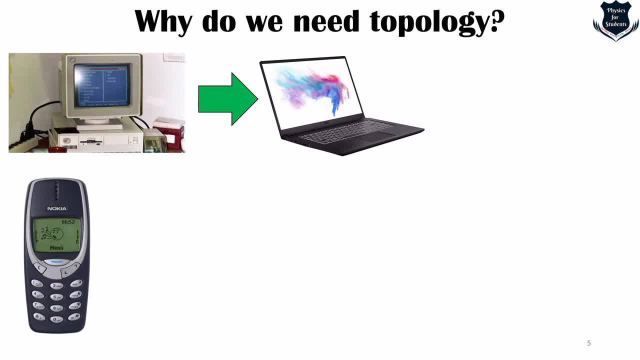 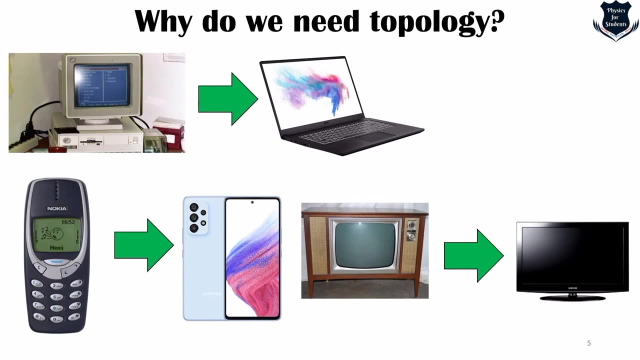 some people you also have. this is a Nokia 3310C, if I am not wrong with the model number. This has now got into a smartphone. The television, which used to be huge in size, now became a smartphone And now we can use the communication for various purpose. We can use mobile not only for talking. 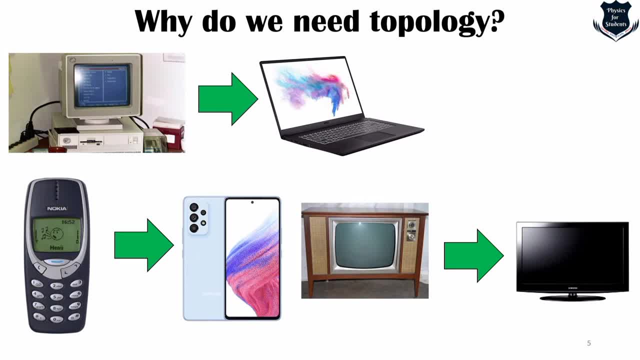 but we can use for telephone, for communication, for messaging, for live videos and everything. Same goes with television and with a laptop. So on a smart TV now we can use pen drives and whatnot. So the bottom line is that these things become more generalized. Obviously, things become. 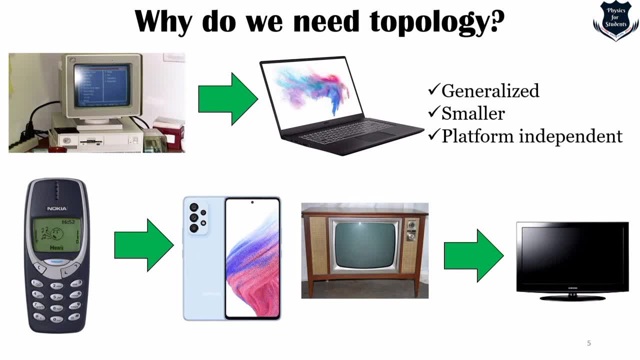 more, smaller And, most importantly, they become flat. So the bottom line is that these things become more generalized. Obviously, things become more smaller And, most importantly, they become flat. DataДаwn, or essentially dataصaan, become more general. That means, if you go with technology, for example CC++, Java, as they moved up the ladder, 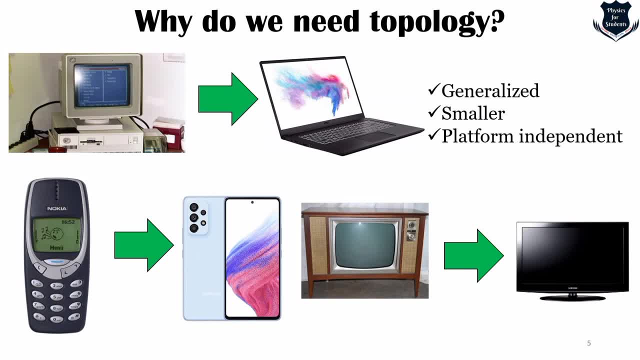 you will see that most of the softwares became platform independent and become browser oriented at the same time, So that it can run anywhere independently without the need of a certain operating system. Topology also serves the purpose of becoming generalized and platform independent, as we will see in the next part of our video. 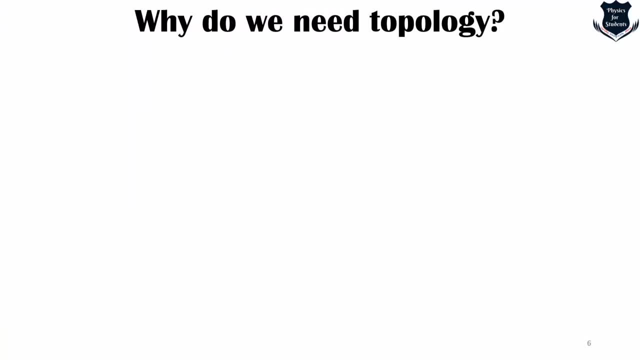 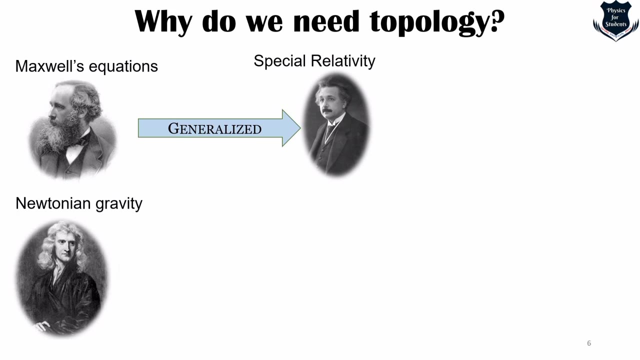 The next video is hablando detable, So this is something which is very important if you consider the development of scientific process. Maxwell's equations was further generalized by Albert Einstein in his special theory of relativity. The Newtonian gravity, which was generalized into a space-time curvature by Albert Einstein in general relativity. 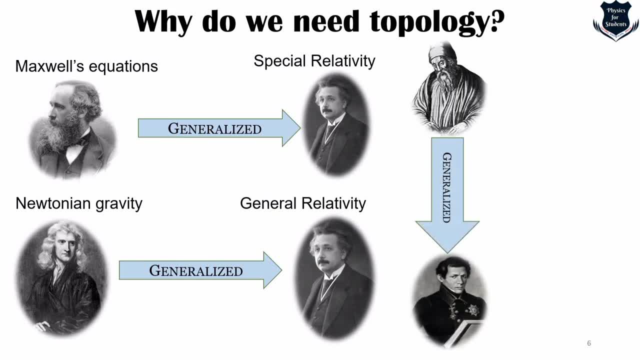 The Euclidean postulates was further generalized into what is called a non-Euclidean geometry by Nikolai Lobachevsky, And the Euclidean axioms got generalized into topological axioms, which is the main purpose of this video. So up till now, what I tried to tell you is that, with the development of science and technology, there has been certain changes. 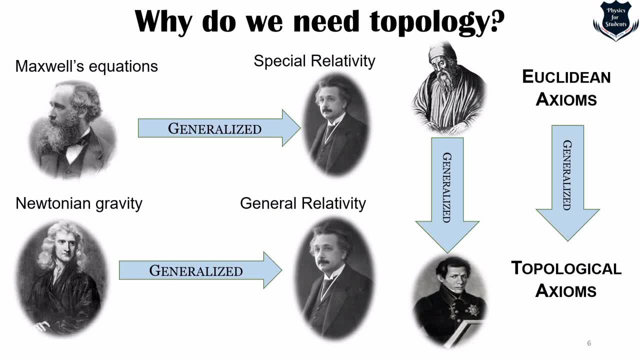 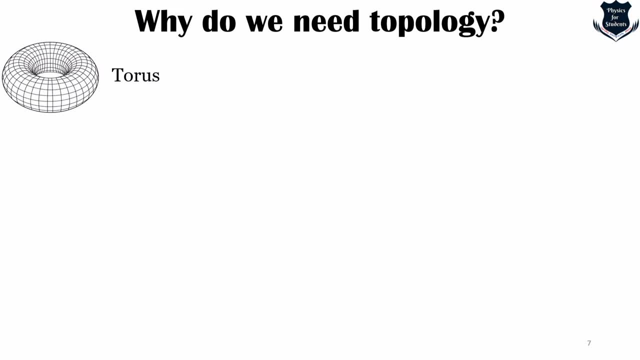 The changes are becoming portable, much more generalized and becoming platform And independent, and exactly that is what topology has done. Now, if you see the shape of the objects- I have shown this in my previous video. also, If you have missed the last video, which is basically on the concepts, and you know basic concepts of topology- 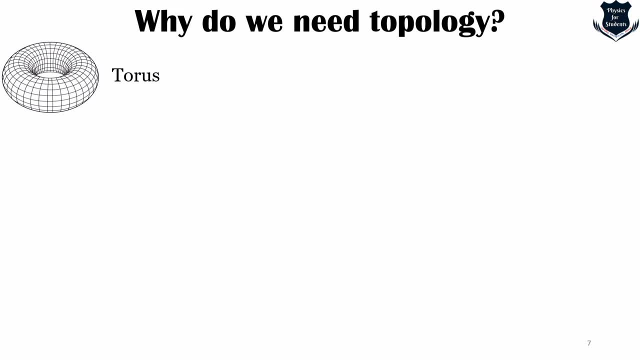 I have given it in the I button. You can just go there and click on it. And the cup as well as this ball. These all can be turned into other shapes like circle or square And a rectangle, or into any kind of a shape. 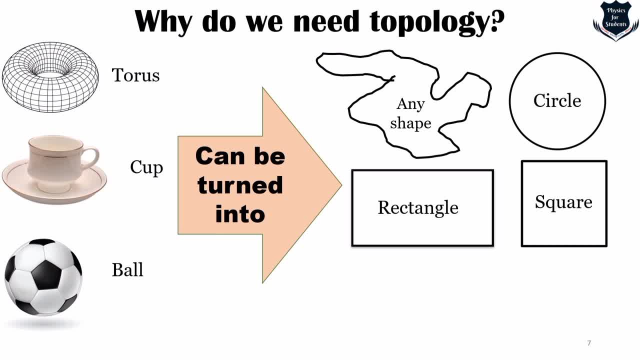 How it has been termed. what is the geometry and what is the underlying mathematics? I am not going into it, But assume that these can be turned using homeomorphism and other technical things. It can be turned into any shape. So what I am trying to tell is that a circle is topologically equivalent to a square. 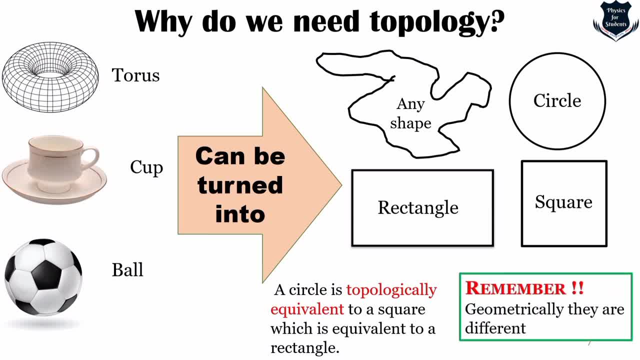 Which is again equivalent to a rectangle. But remember that they are geometrically they are the same But topologically they are different. I mean to say that topologically they are equivalent but geometrically they are the same. So topological equivalence doesn't mean that geometrically they have to be equivalent. 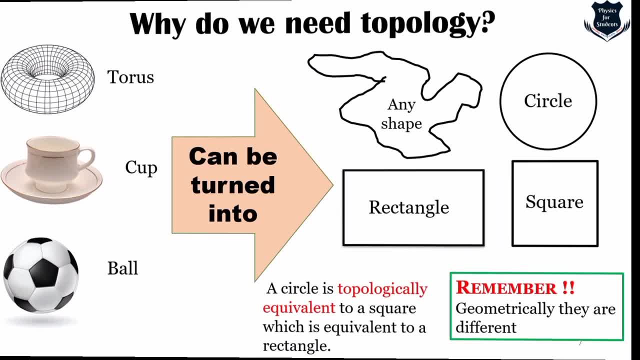 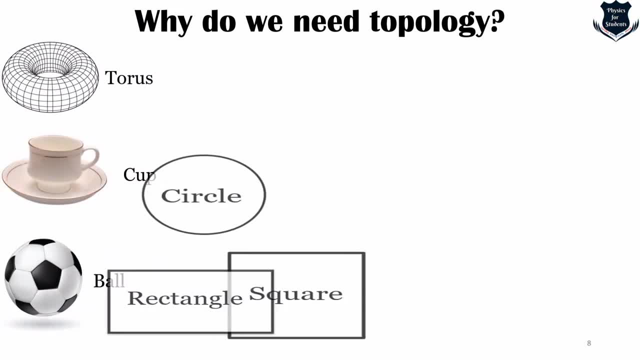 But remember that geometrically they are different. Now, if I go into the next part of our video, What I am trying to show is that this torus, this cup and this ball, when they turn into circle and rectangle and square, Are generalised into any kind of a shape. 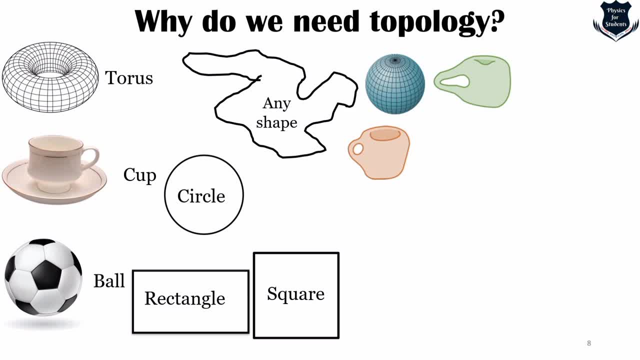 Then these takes form of a cup, of a sphere, and this kind of shape, a torus, Or a torus which has got three holes. that is called genus three. So the basic idea, what I am trying to tell, is that it takes any shape. 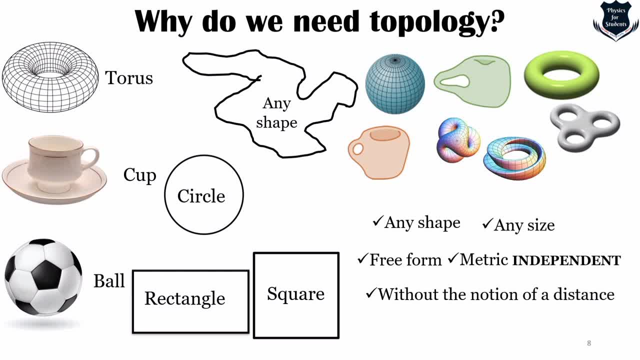 It takes any size. It is becoming a free form. That means I can change these structures into anything. It becomes metric independent. That is the most important part. That means I do not have to measure. Definitely I am going to measure, But I am not going to measure those distance or the angles or whatsoever on a particular metric. 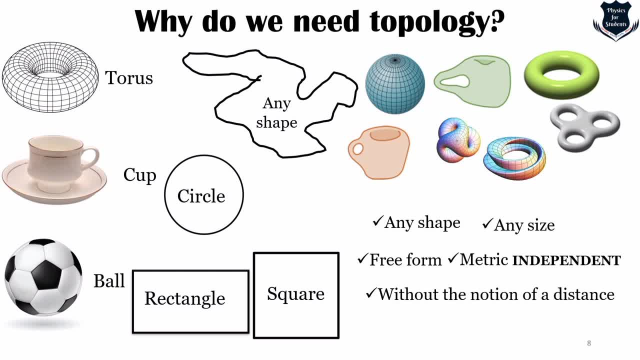 That is a meter or a centimetre or whatever. The metric will become independent and without the notion of distance. Now, what do I mean by the notion without the notion of distance? That will come in the next part of our video. So once we see these shapes, 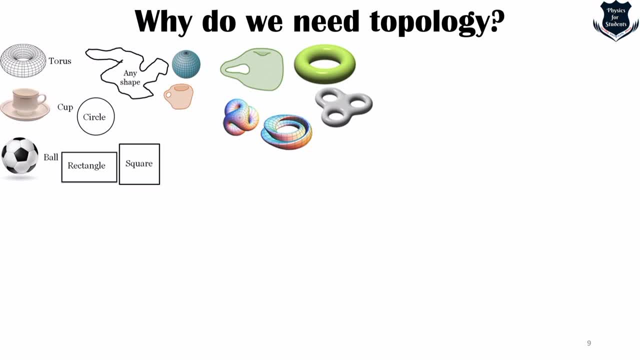 Are Deformed into any other shape. It can be Euclidean, Cartesian coordinate shapes, It can be non-Euclidean shapes. But if I take all those shapes and if I deform them by stretching and bending- And there is definitely certain tool, 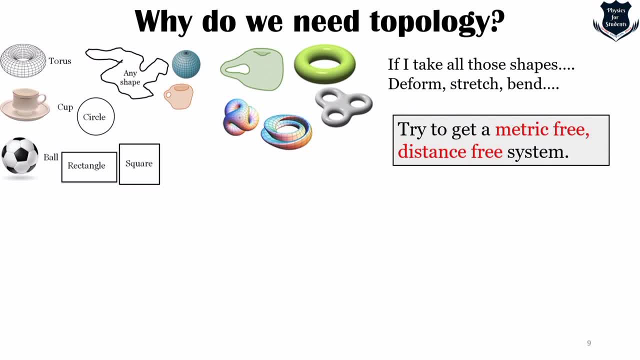 Then why I am doing is that I am trying to get a metric free, distance free system. That means I am not going to depend on any specific metric or a specific distance, Which we call it as distance, But the measurements will be invariant. I have talked about topological invariant in my last video. 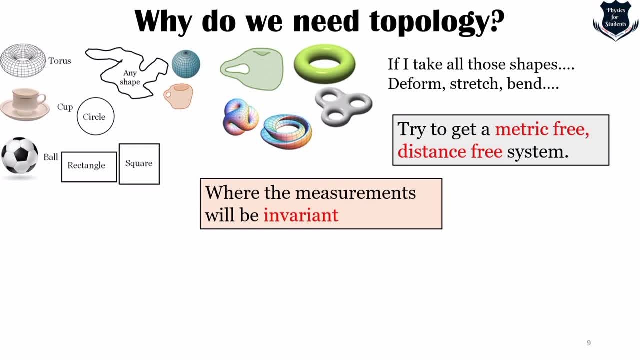 Which you can see in my playlist. So the basic purpose is, just like technological advancements, Mobile is no more a mobile, It is serving further purposes. Television is no more a television, It is serving multiple purposes. So it is become television mobile. all this technology has become metric free. 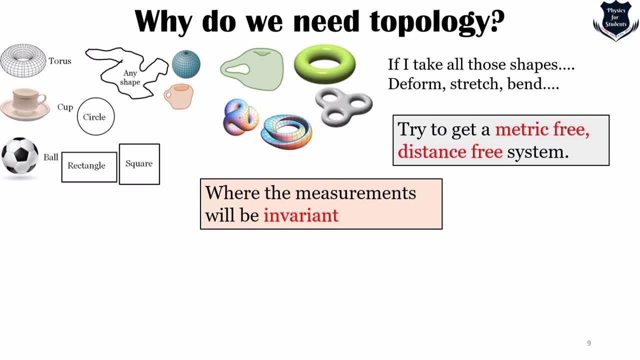 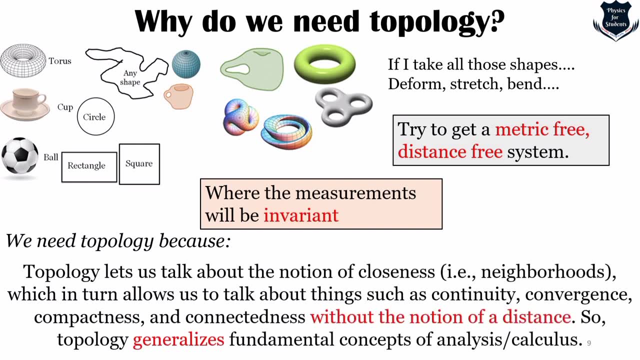 But the measurements and the purpose is the same. Same goes with topology. Here comes the reason that. why do we need topology? So, in topology, because it talks about the notion of closeness, Which is technically called Babel rules, Which in turn allows us to talk about things such as continuity, convergence, compactness and connectedness. 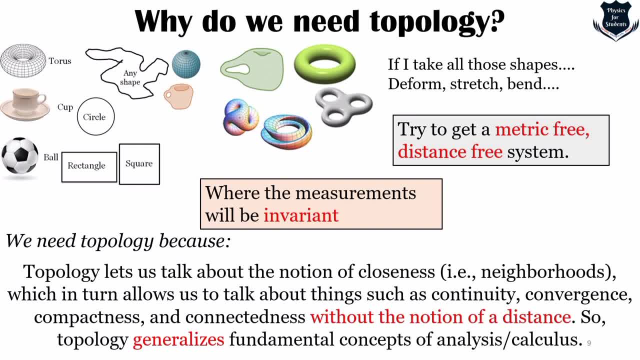 Without the notion of distance. So topology generalizes fundamental concepts of analysis and calculus. So if you look closely into the topology, The definition below, That means the topology is going to generalize certain concepts And the continuity, convergence and connectedness. 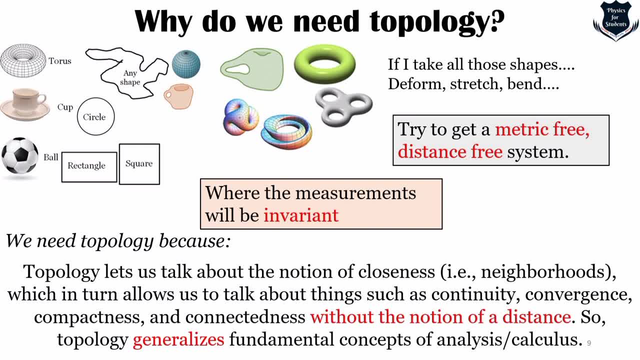 These will definitely be there, But without the notion of distance. Why without the notion of distance? Because distance means we are depending on a specific metric And whole purpose of technological advancement is to become metric free, And topology is not an exception. So now we will see that how these distance or measuring free will become clear to us. 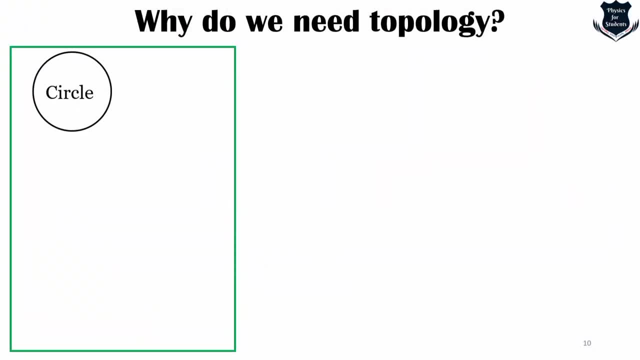 Now, if we take these shapes- I mean to say normal shapes, Which are Euclidean shapes, For example, if I take a circle, a cube, a rectangle and a square, And if I take even a triangle, Then what we can see is that there is another set of, you know, deformed objects or non-Euclidean shapes. 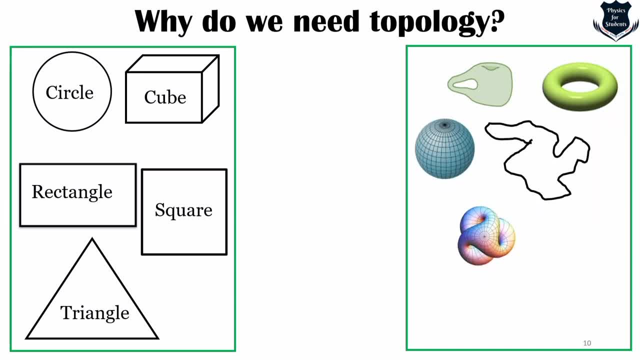 Like a torus and a cup, Or I can take a sphere Or any other different kind of shapes which emerges. So you have one set of, you know, shapes which are typically Cartesian or typically Euclidean, And you have another set of shapes which are non-Euclidean. 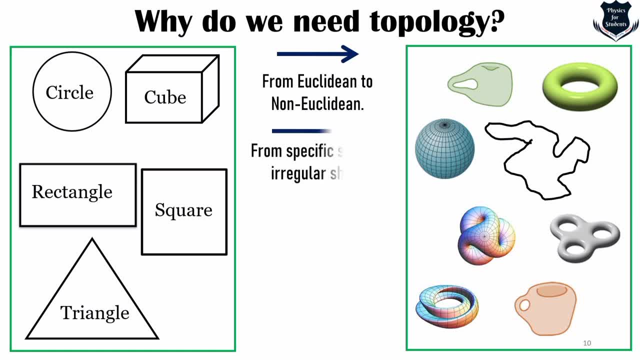 So what happens is that we move from Euclidean to non-Euclidean. So from specific shapes we are now moving into irregular shapes. Why we are making irregular shapes, We will soon see that. So from Euclidean axioms, definitely we need topological axioms. 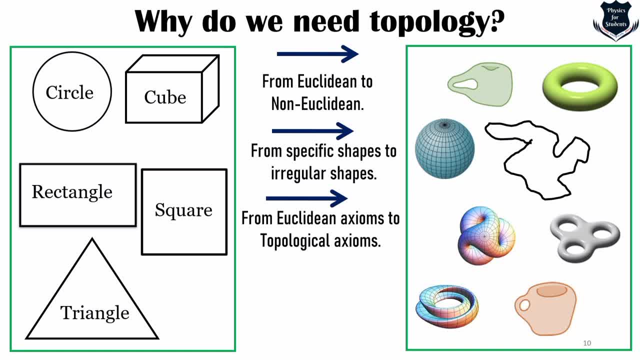 Because Euclidean axioms in specific shapes won't work in irregular shapes, And also from metric system, we are moving into a broader system which is called a topological space. So up till now, what I tried to show you is that, as far as the technological advancement and things are going in advanced nature is concerned, 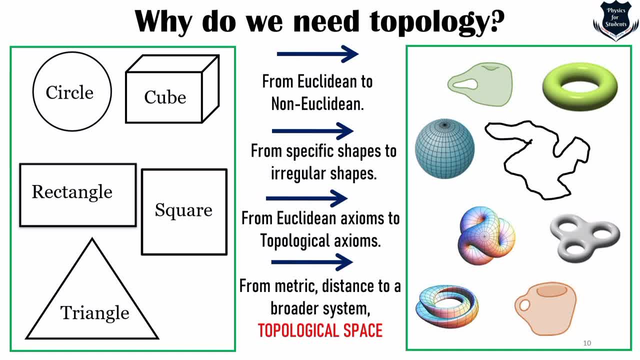 The topology is also an advancement in terms of human thinking that we are generalizing And we are trying to get something which is called, you know, metric free, And for that we need a different kind of a system, And for that we need a different kind of a space. 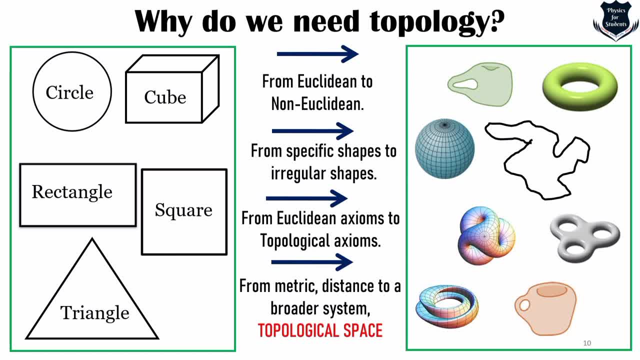 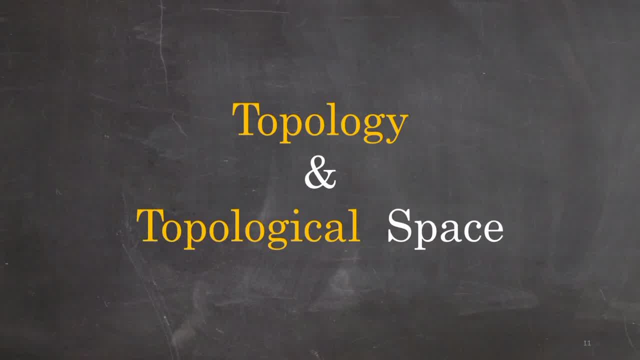 Why? Because the Euclidean and the Cartesian rules won't be allowed in the space. How do we form that kind of a space? That is coming up, That is coming up in this part of the video When we talk about topology and topological space. 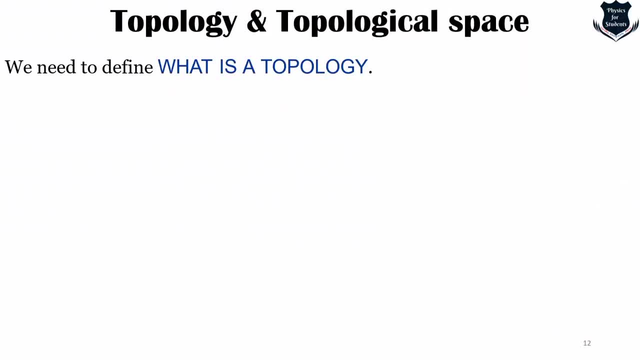 So Euclidean space First, what we need is that we need to define what is a topology. Okay, So once we define a topology, we study in general. if you look, it is called a study concerned with the shape of geometrical objects. 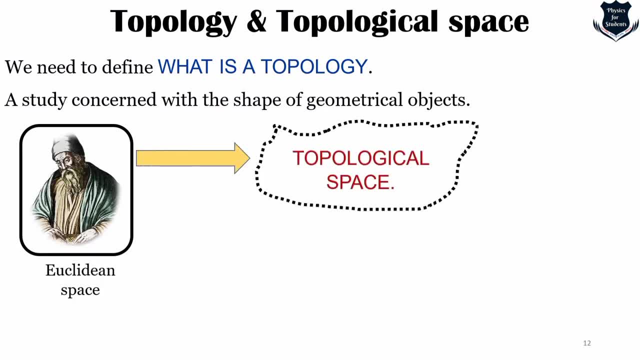 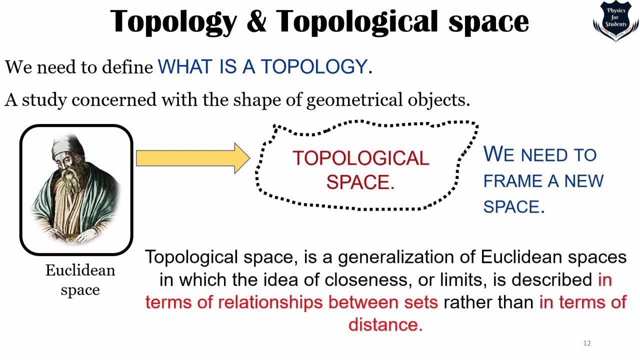 So, from the Euclidean space, what we are trying to do is that we are moving into topological space. Why? Because we need to frame a new space, a new set of rules that these geometrical or deformed or different type of weird objects will take place. 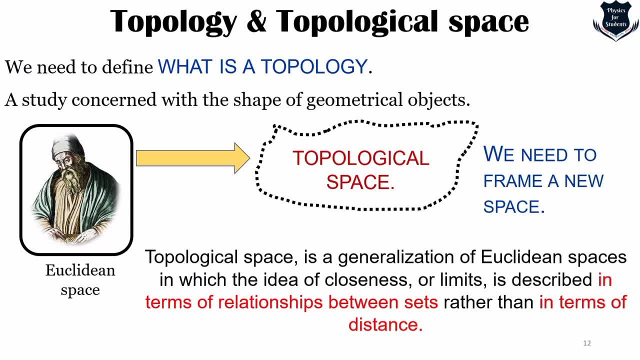 So topological space is a generalization of Euclidean space, in which the idea of closeness, limits, is described in terms of relationship between sets rather than in terms of distance. So here comes the basic crux of topology and topological space. 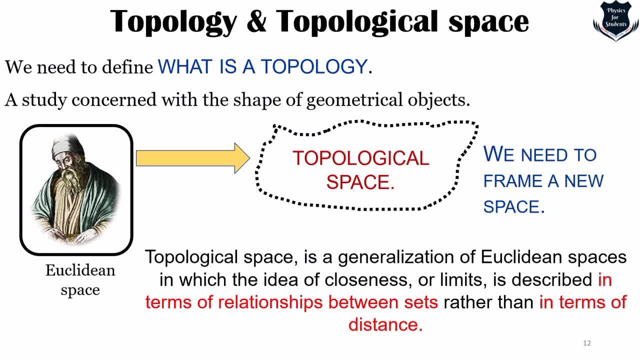 That we need to form a kind of a rule that all these things will be measured, but in terms of relationship between sets- And that is why set theory is predominant in working out topological mathematics- and in terms of distance, We won't measure in terms of sets. 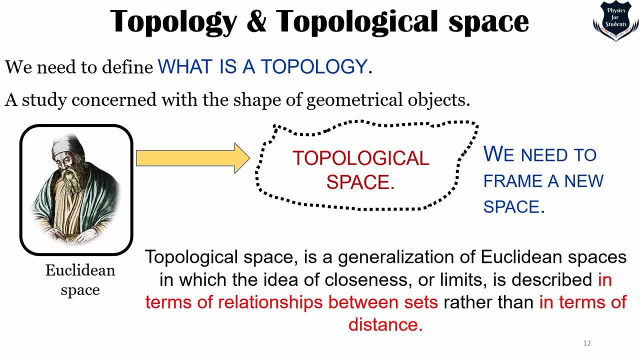 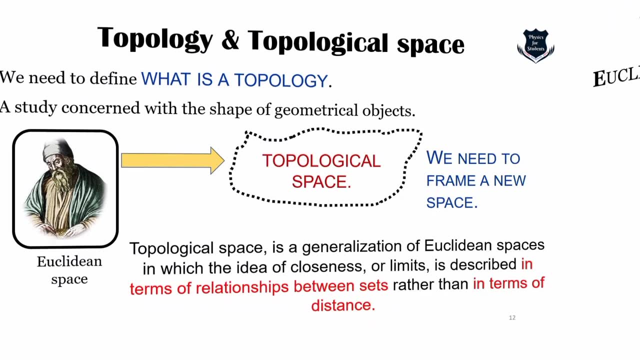 Set theory being the predominant mathematics of topology. Okay, Helps you to give a much more broader scale. Differential geometry, being a local candidate, looks into differential calculus, But here we are dealing with much more broader forms, So what we need is a topology. 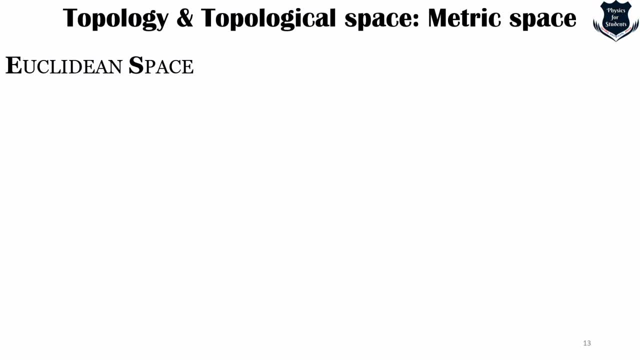 Okay, First we will quickly define what is a Euclidean space and get a basic concept so that the movement would become smooth. So Euclidean space is basically the fundamental space of geometry. Euclidean geometry intended to represent physical space Originally, that is, in Euclid's elements. 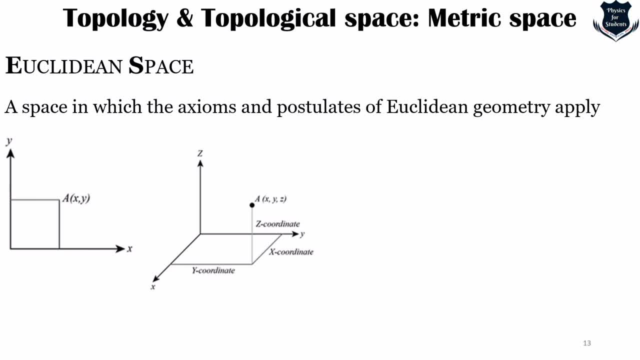 It was a three-dimensional space of Euclidean geometry, But nowadays you will see in modern mathematics there are Euclidean spaces of any positive integer dimension. The qualified Euclidean is used to distinguish Euclidean spaces from other spaces that were later considered in physics and modern mathematics. 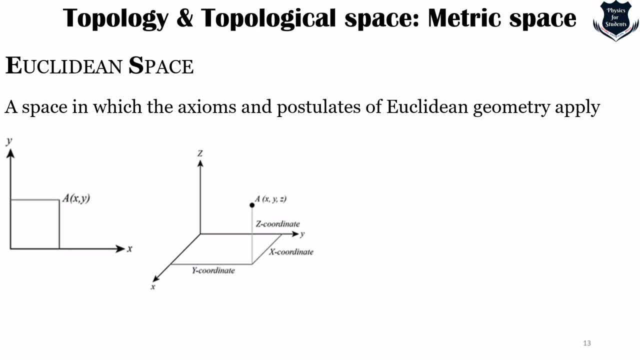 Right on your screen you can see a kind of a schematic diagram of a Euclidean space, And from Euclidean space we go into metric space, set together with notion of distance between its elements, usually called points. So in Euclidean space we measure points. 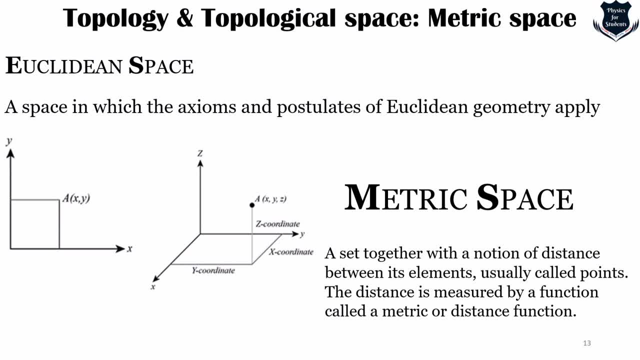 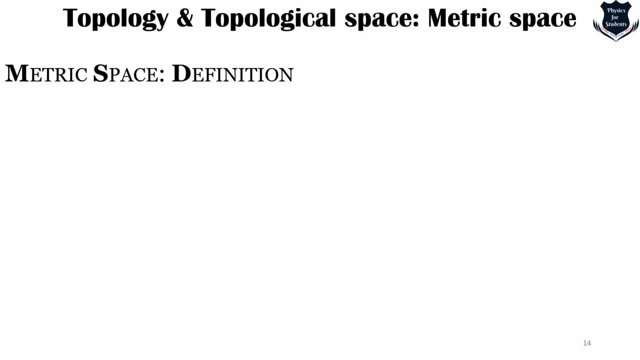 But in metric space this distance is measured by a function called a metric or a distance function. So in metric space definition, If I talk of the definition itself, Metric space is a set, together with a notion of distance between elements called points. The distance is measured by a function called a metric or a distance function. 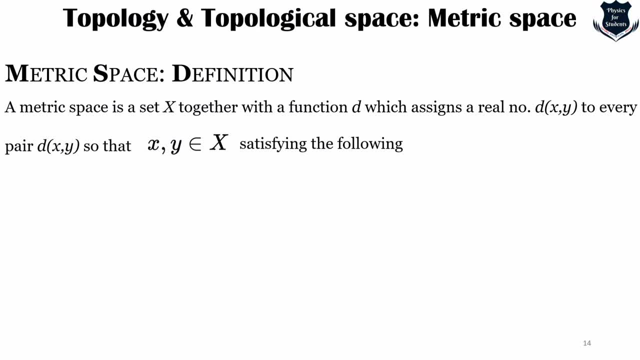 Metric spaces are the most general setting for studying many of the concepts of mathematical analysis and geometry. So here you see, if a metric space x together with a function d which assigns a real number, Or if a metric space y and x are same, then this is X or Y, which shows that X and Y are relevant, of X which satisfies 1.. 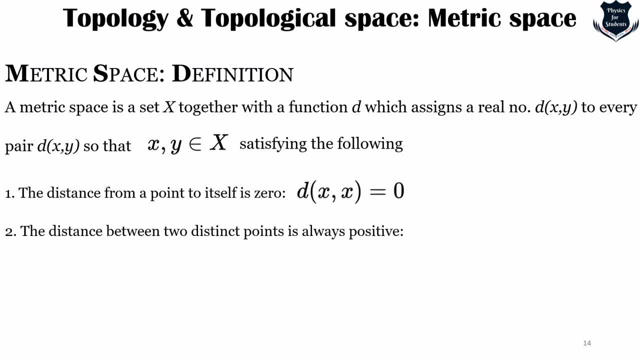 The distance from a point to itself is 0. Which means this: The distance between 2 distant points should always be positive, So it should be greater than 0. And the distance from X to Y is always the same, which means this one: 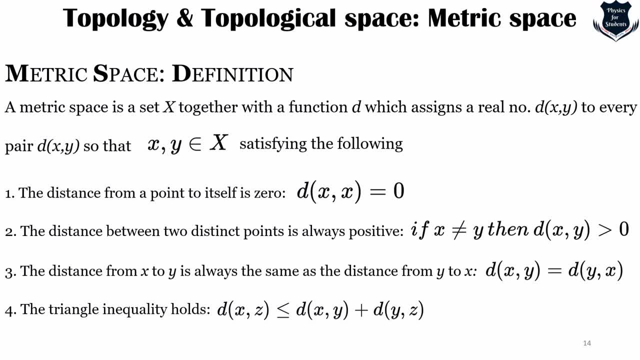 So X and Y and Y, X are the same And it obeys the triangle inequality. So this is how the metric space definition is important, that we are using, most importantly this t, which is a metric or a distance function. So why we are mentioning all those metric? because now you will see how the migration 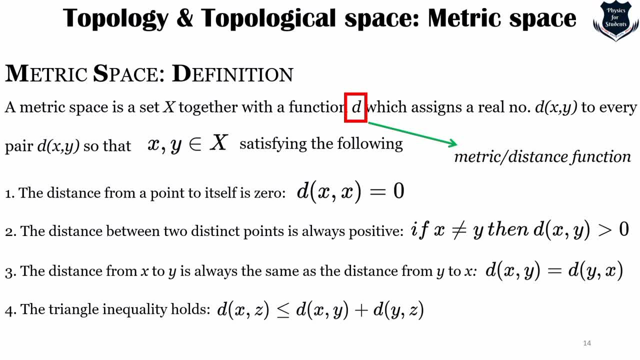 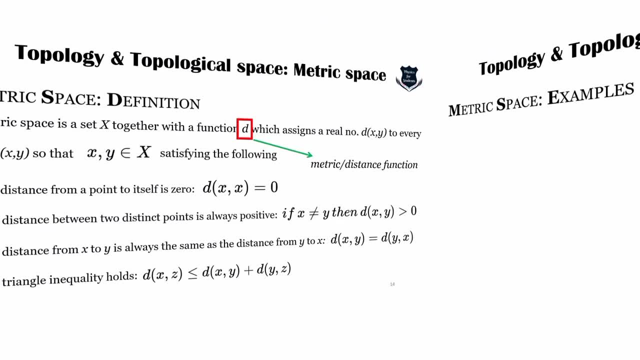 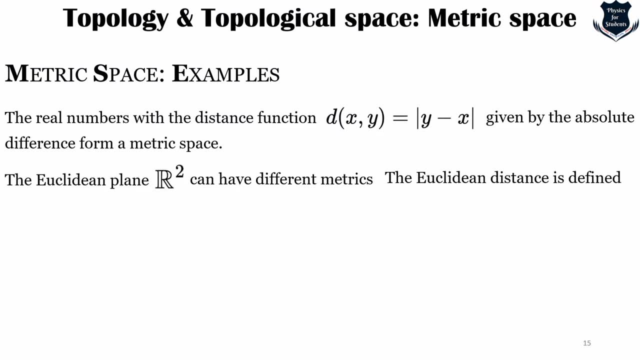 becomes more So. till up till now, metric space definition is using the function t and it obeys 1,, 2,, 3 and 4th triangle inequality conditions. Okay, let us see quickly some examples of metric spaces. The real number of the distance function gives the absolute distance. 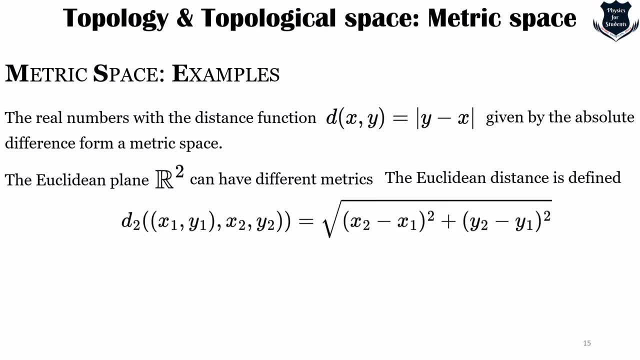 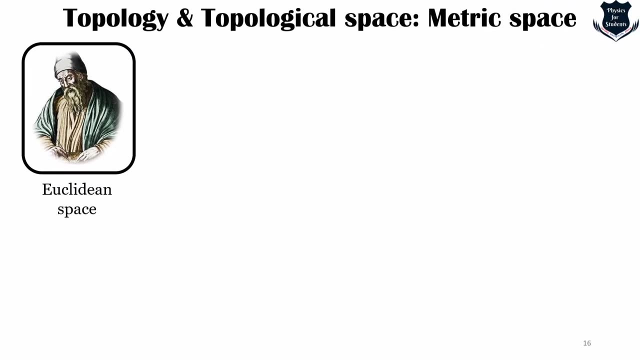 Euclidean space R2 can have different metrics, for example this one: The taxi cab distance is given by this one. I have not shown Euclidean distance because it is too rudimentary and can be understood by any class going school going person. So these are some of the examples of metric space. 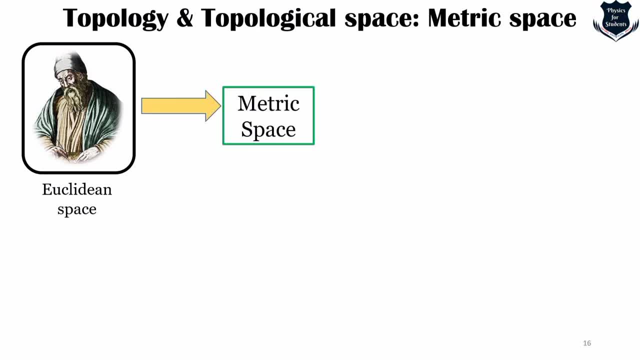 So where have we gone? So, from Euclidean space we have moved into metric space, Which is the real numbers and it measures with the distance function, t, and now we move into something which is called a topological space. So, topological space, it generalizes the structure set in Euclidean space. 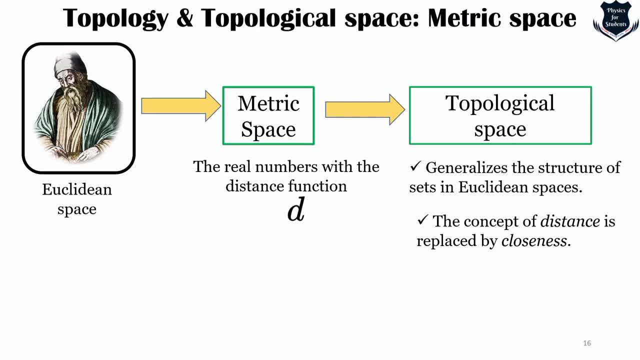 It the concept of distance- now, we won't call it distance between two points, we call it closeness- and a space where those elements of set are called points. It is a most general type of mathematical space That allows the definition of limits, continuity and connectedness, and it formalizes the concept. 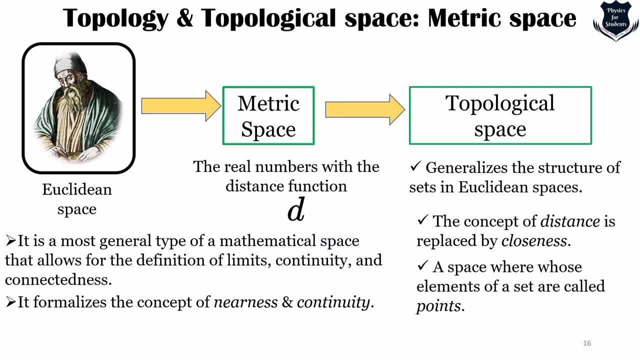 of nearness and continuity. So, brief, up till now, this is how the migration and the movement takes place. So from Euclidean we move to metric, which is where the distance is measured by a function, and now this distance is measured by closeness and a space where these elements will be there. 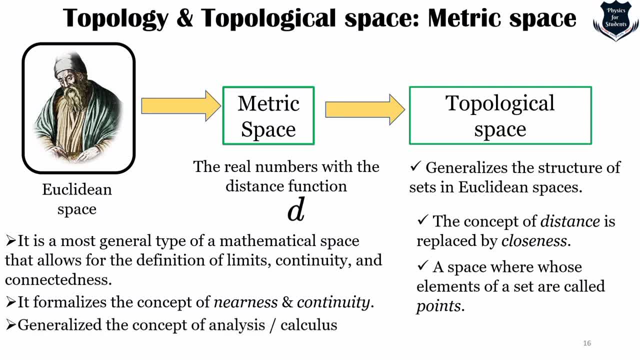 these will be called points And, most importantly, Right at the bottom of your screen, generalizes the concept of analysis and calculus. So, whatever we are now doing, as you see, it is constantly generalizing, making things broader, making things easy, and that is why it is portable. and, as you see, I started with the history. 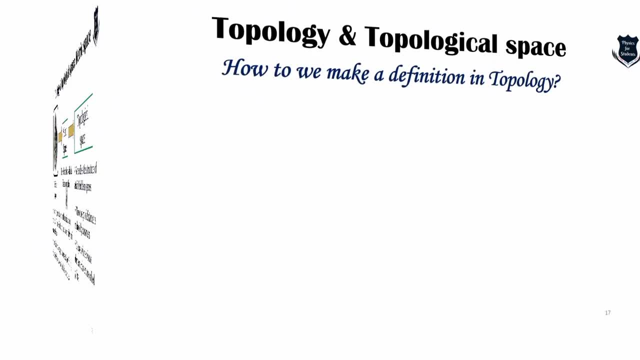 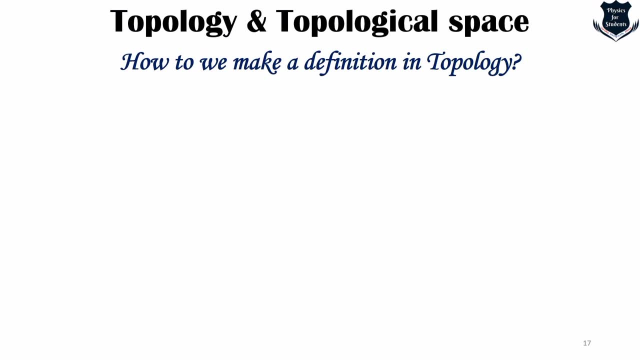 of technological advancement. topology is also the same. Okay, so first is that, how do we make up a definition in topology? Now, you see, when we talk of a definition in topology- I would like to use an analogy- that there are certain characteristics which, if an object or a specific genre that specifies 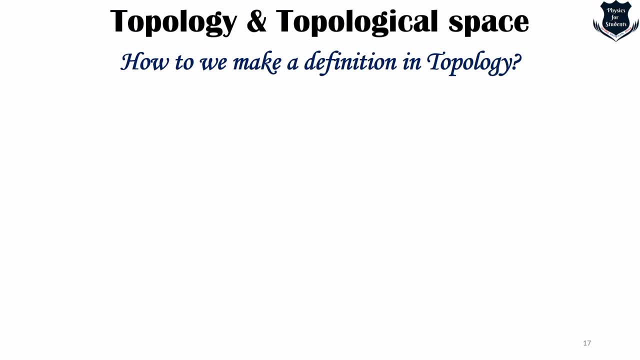 or they have, then we name that object or genre something else. For example, if I take a frog, Okay, in general frogs have a protruding eyes, no tail and strong- you know, webbed hind feet that are adaptable for leaping and so on, Leaping and swimming- and they also possess a smooth, moist skin. 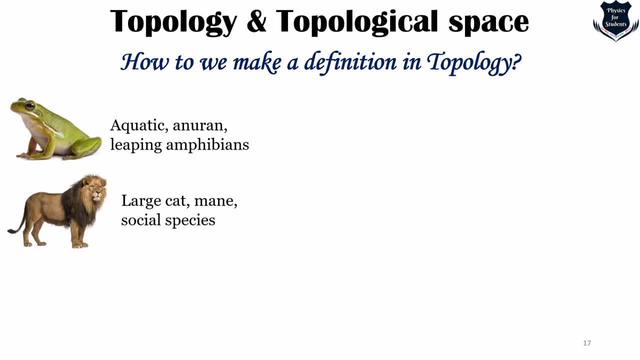 So these are the characteristics which makes up a frog. So lions similarly have strong, compact bodies and powerful four legs. teeth and jaws are pulling down and killing prey. something like this. Even you know a tiger, you would be warm-hearted. you're fearsome, you know courageous in the 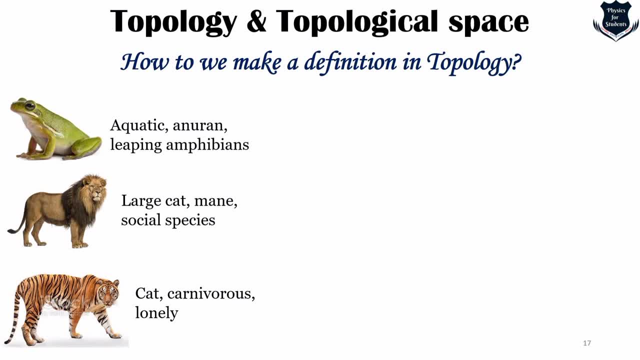 face of a danger, yet yielding and soft and mysterious- All those characters. So, if you see a lion and a tiger, we cannot say each of them are of the same. why? because each of them has a specific characteristic right. So, as I told that lions have to be strong, compact, this is this, and a tiger has to be. 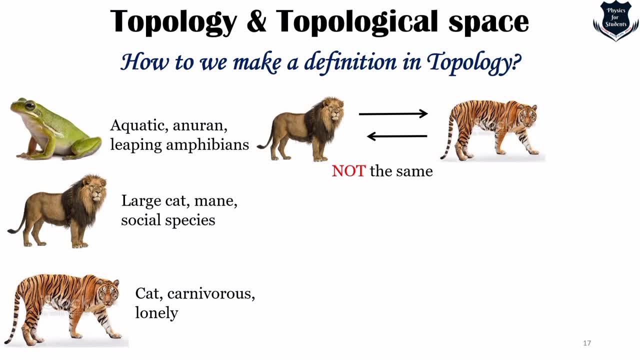 this, this, this and aquatic animal has to be this, So that is why these cannot be the same. So topology, like other branches of pure mathematics such as group theory, is an axiomatic subject. So what do I mean by axiomatic? that is the definition. 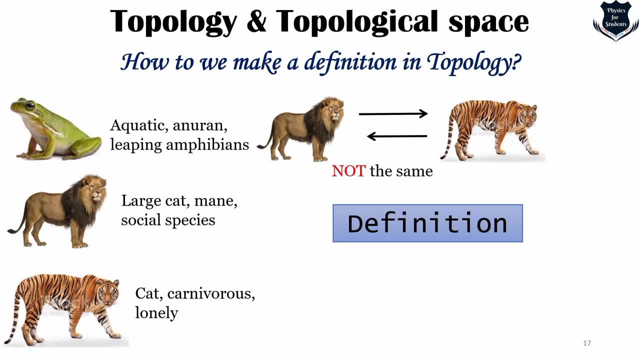 So we start with a set of axioms and we use these axioms to prove propositions and theories. So a definition: it should be there and it should certainly satisfy certain conditions, and then we call it that: OK, this definition is true or false or whatsoever. 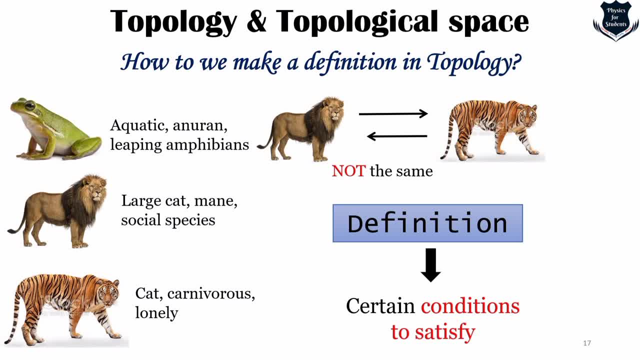 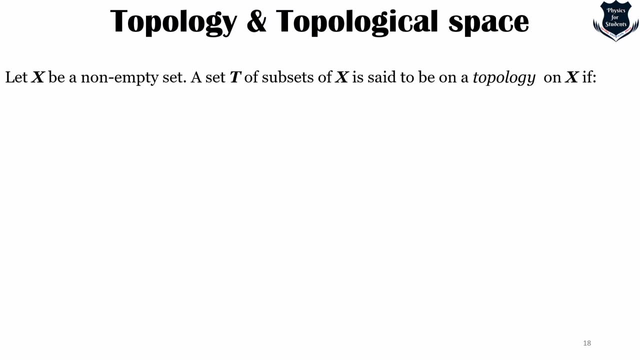 So this is how we make up a definition in topology: that it has to satisfy certain characteristics. So I just tried, I tried to give you an example with these. you know animals and so OK, So what is a topology and what is a topological space? 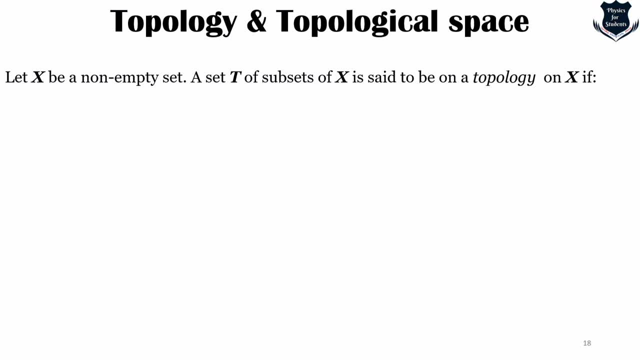 So first let us see that if X be a non-empty set, don't worry, I will just give you a visual aid. a set of T, of subsets of X, is said to be on topology, on X. If that means, what are the conditions? 1, X and the M sets. 5 belongs to 2, T, 2, the union. 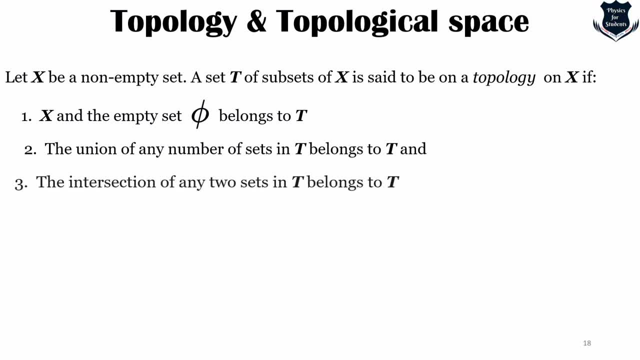 of any number of sets of T belongs to T and the intersection of any two sets in T belongs to C. So now let us see how we can demonstrate it visually. Now this sphere X and T is called a topological space. Now here is a set, X, here is my subset, T, and if I consider 5 to be empty and X is a non-empty, 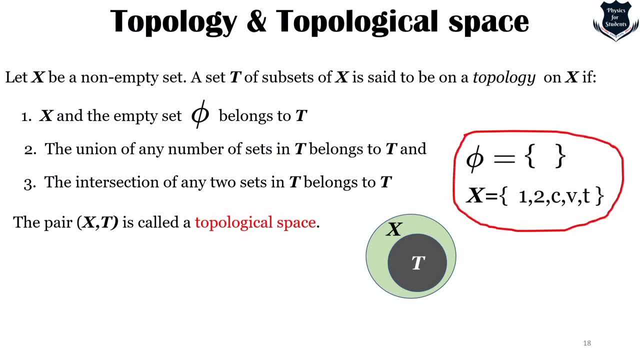 set. So I just given any random numbers: 1, 2, etc. This is what this is Right. So X and the empty set. this Now, as because it is saying that any number of union of sets in T belongs to T. So I have just measured, named it: set 1, set 2. any number of you know the union. 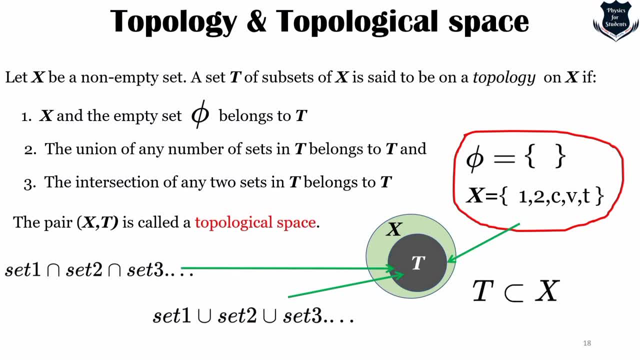 So yeah, So the intersection, as well as the union, all of them belongs to T, and this is just a mathematical thing. This entire part, the sphere X and T, is called a topological space. I hope so from the mathematical definition, what we have seen, that X and the empty set. 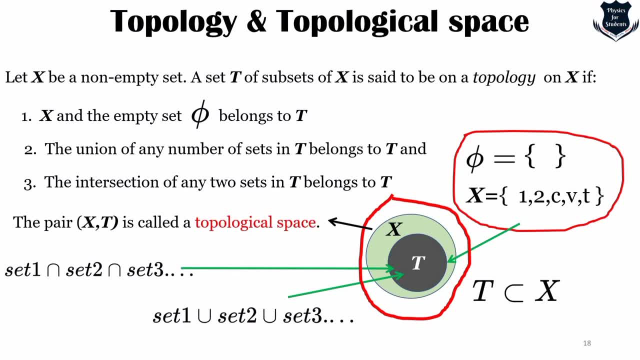 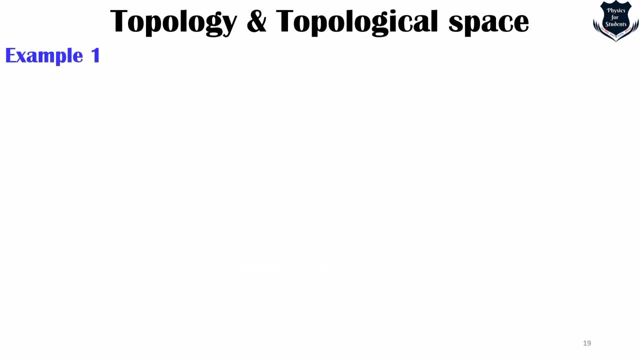 5 belongs to T. This would give you a better understanding that what I is, what X is, an empty set, and how the set intersection and the union belongs to T and this entire figure, which is in red marked, is called a topological space. Few examples would make things clear. 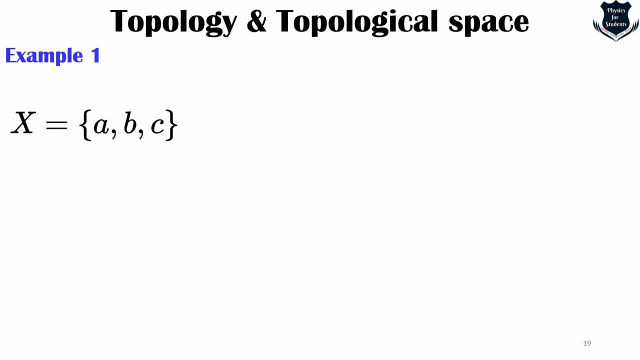 So now let us see. For example, Let us take X equals to ABC. Now what I am trying to do is that first I am going to give you a visual demonstration of what is a topology, and then I will come to the mathematical part. 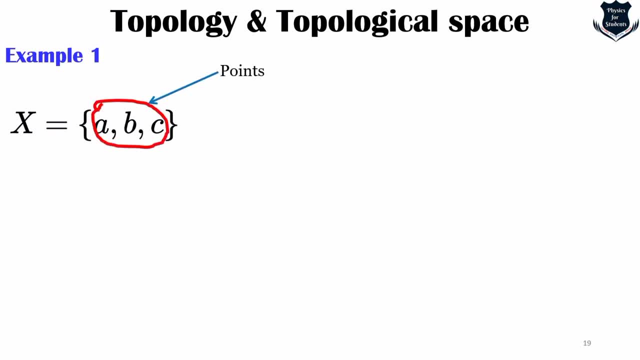 So ABC means we have learned that these elements in the set is are basically points. So let us see if I take a set like this and ABC, this can be one topology. Again, I said take a set round like this, So the subset and I take this one can be a topology. 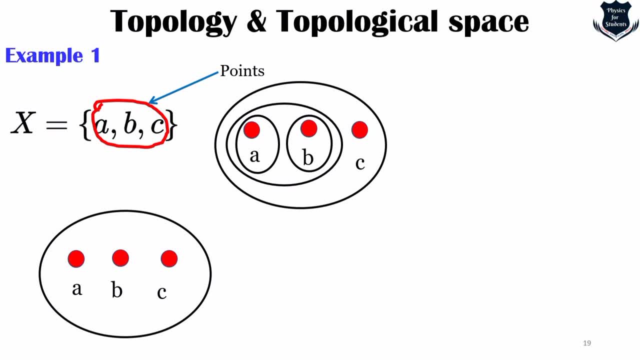 This one and this one- this can also be a topology- and this one the subset A and B. this can also be a topology. Let us say again: we take this one and then we form this one and BC also taken together. again we see A and then we take C, B and C. this can also be a topology. and then again: 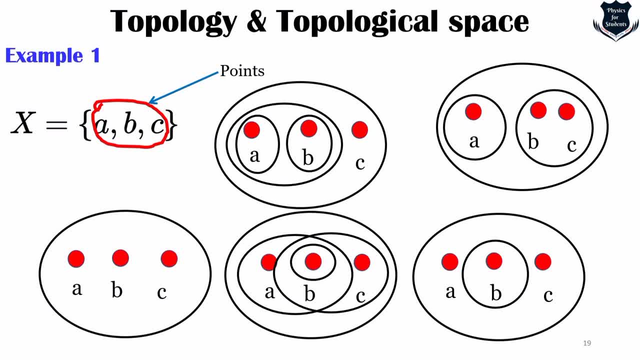 we take A, B and C and within that we form another B subset. this can also be a topology, So I just tried to show you that when you will be going with mathematical examples, these comes as a very important part. So taking X equals to ABC, which means that these are the three points. we have shown how. 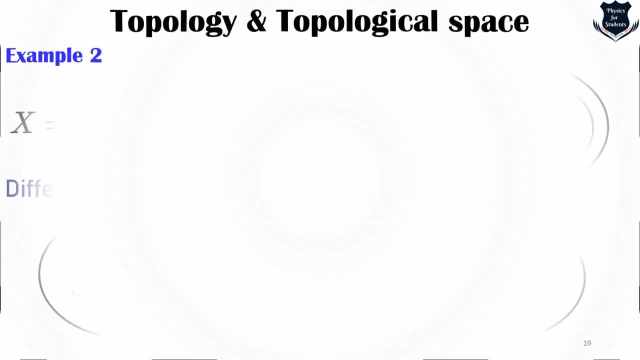 different topologies can be formed. Now let us look into the language of mathematics. but pretty easy. So if we take X equals to ABCDEF and T1, say, for example, we take those two points- You know values- then first one, the X and the empty set phi. let us see X and the ABCDEFI. 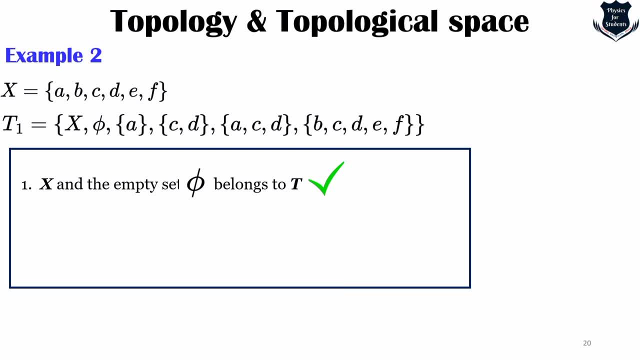 yes, it belongs to T, so this condition is satisfied. Second, the union of any number of sets T belongs to T. you can count those elements, you will find this also satisfied. and the intersection of N to sets T belongs to T. you will count and you will find these also satisfied. 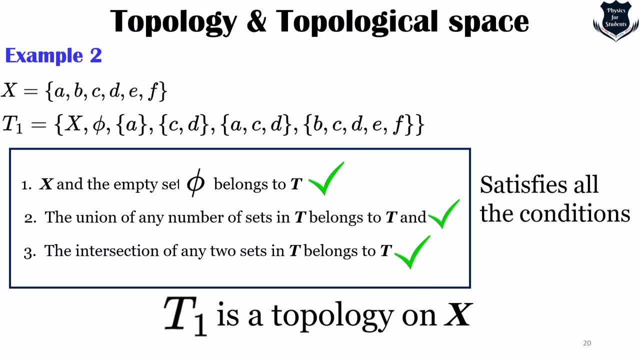 So once all these conditions are satisfied, I can call it: T1 is satisfied. This is a topology on X. So these are how. this is how we do. So we give a kind of a figure or a number and then we go one by one. apart from the definition, 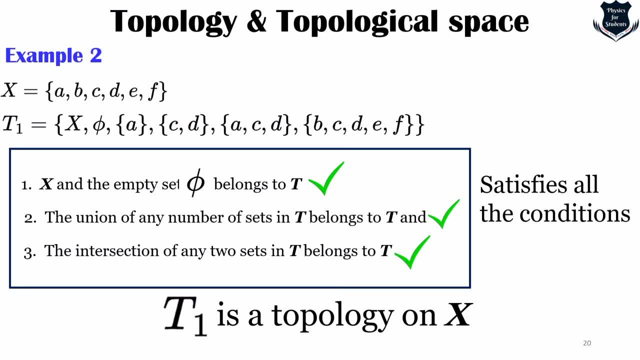 it is satisfied, dissatisfied, dissatisfied. then we can call it: If one is not satisfied, rest is satisfied. we do not call it as a topology, as we will see in further examples. So now you can understand that, just like lion and cat and tiger have different specific. 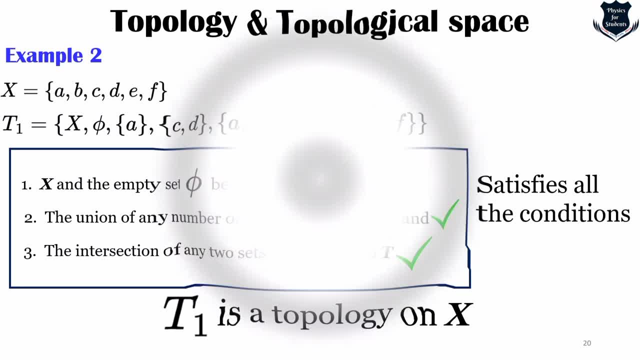 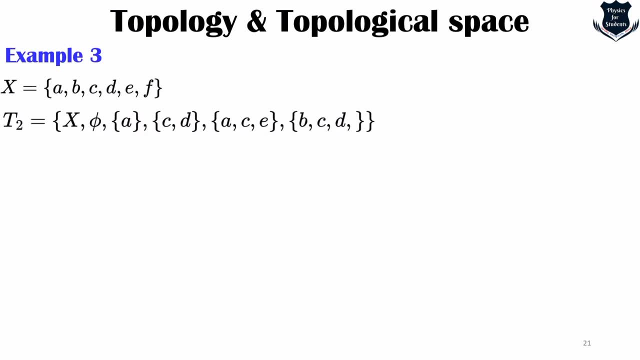 conditions in order to give it a definition. so is topology. Let us see another example where we get the values a little bit different, right? So now let us see whether it values X and the empty set phi- yes, it does. the union of any number of set, does it? no, it doesn't. 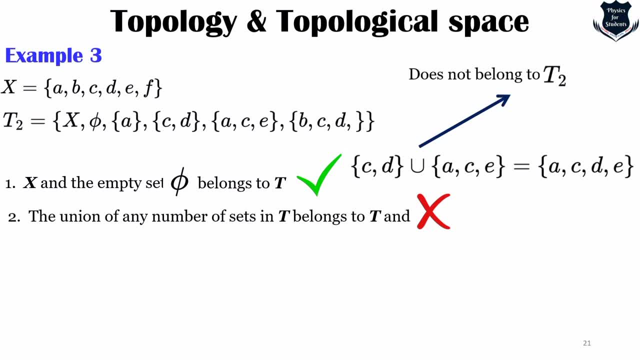 Why? because you will see, if I form the union right- ACDE, and then union of ACE, then the two members T2 does not belong to T, That is, T2 does not satisfy the condition. that is why T2 is not a topology. on X, although. 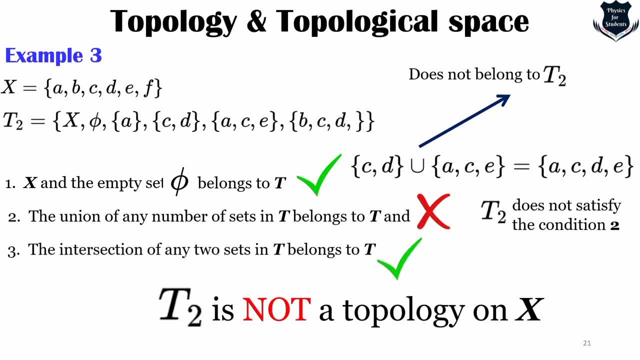 the third condition is being satisfied. So I was just telling that if one of the conditions not satisfied, here you can see that T2 is not a topology as the union of this CD, ACE and this one, two members of T2, this one, C and D, these two members. 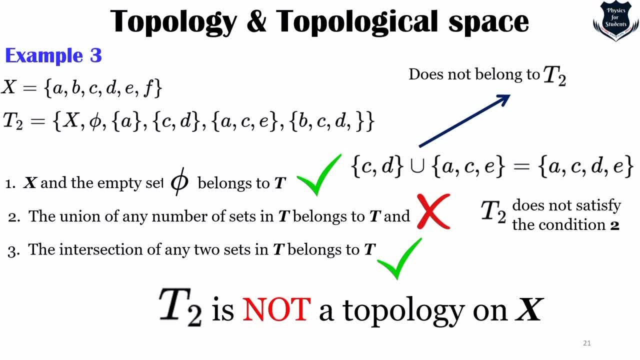 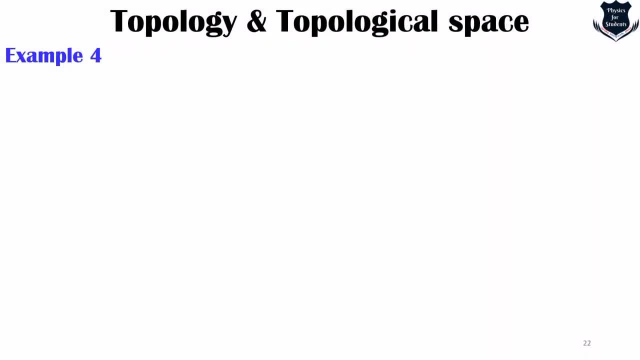 Does not belong to T2, so they satisfy not the condition and hence it cannot be called a topology. on X. Further examples will make things further clear. let us say we take this example where the numbers again are different. then is X and the empty set phi belongs to T. 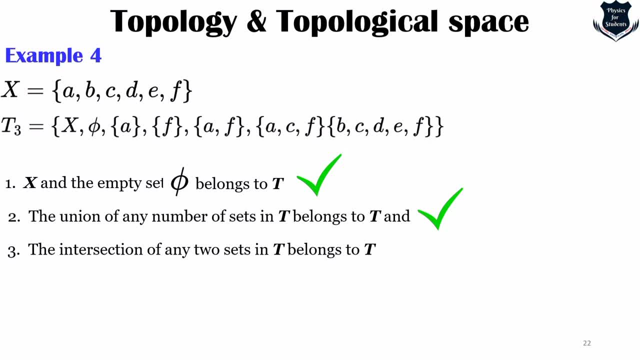 Yes, it does. this does yes, but does the third point satisfy? the intersection of any two sets in T belongs to T. No, Why? If you do a little bit of calculation, you will see that T3 is not in topology on X. Why? because this union does not belong to T3 and it doesn't satisfy the condition. hence, 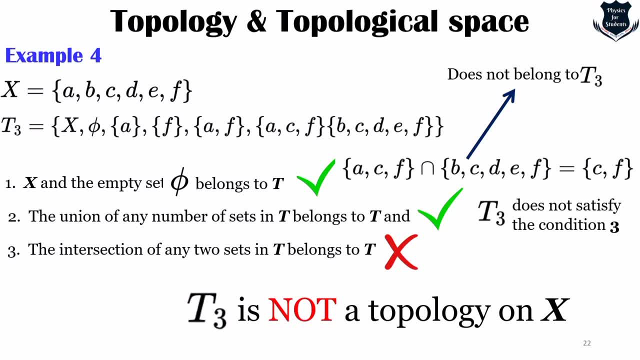 T3 is not a topology on X. So this is the way, this is the procedure, one by one, as we take forward and we understand which one is on topology and which one is not on topology. we need to understand and we need to go through these type of. 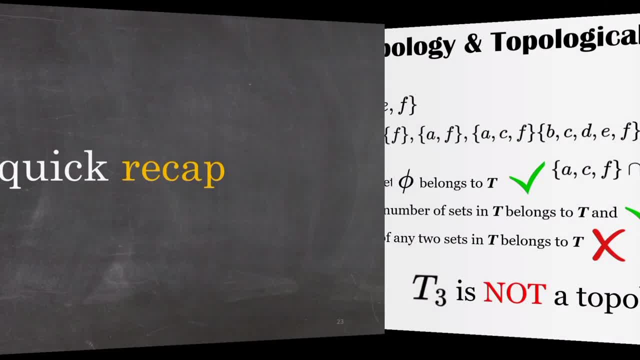 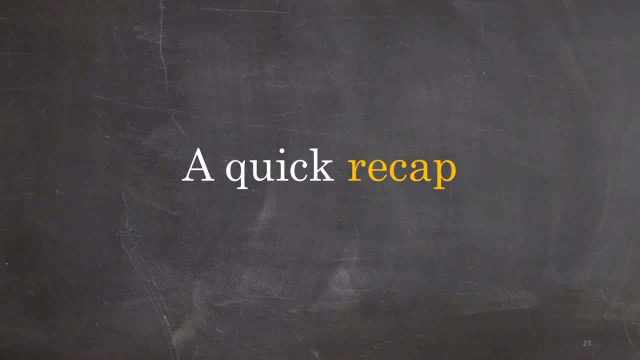 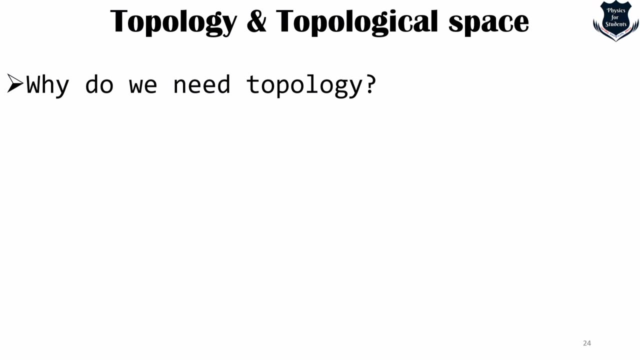 Definitions and their part. ok, so before we leap ahead into the next part of our video, I would like to get a quick recap what we have done till now. so first we have looked into why do we need topology? because of the advancement, because of making things much. 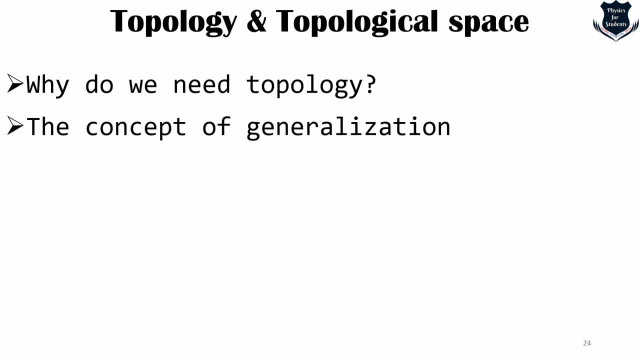 more, broader, easier. we need that, and the concept of generalization is the central the we need a separate space that is called a topological space, Euclidean space. from there we move into metric space And we have also understood what is a topological space and what is topology. 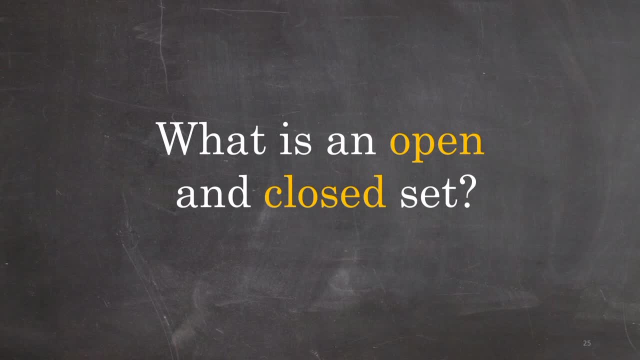 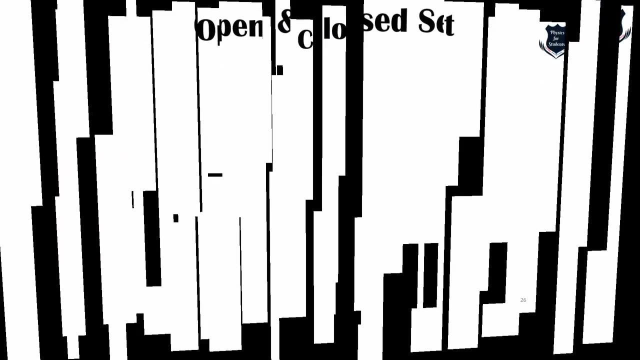 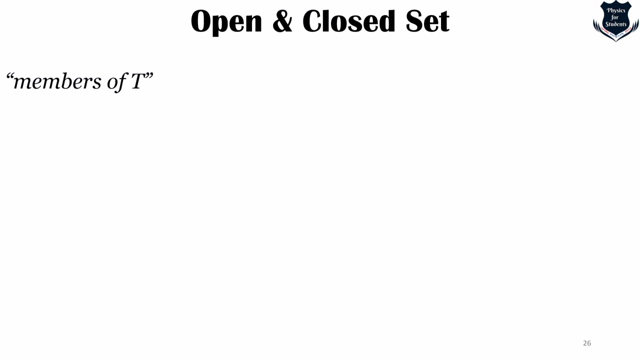 So time to move ahead into the next part of our video, which is very central, and what is an open and a closed set. ok, so instead of telling things like these are the members of E or these are the members of something, we find a more convenient way to give such 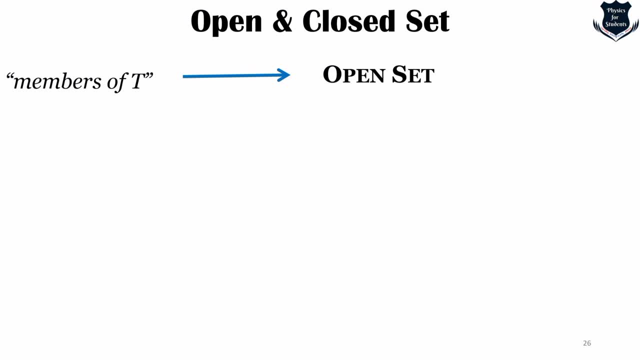 sets, a name We have also complemented. we'll come later. so, more generally, one defines open sets as the members of a given collection, of a given set, a collection that has the property of containing every union of its members. we will see that. so open set is a generalization of 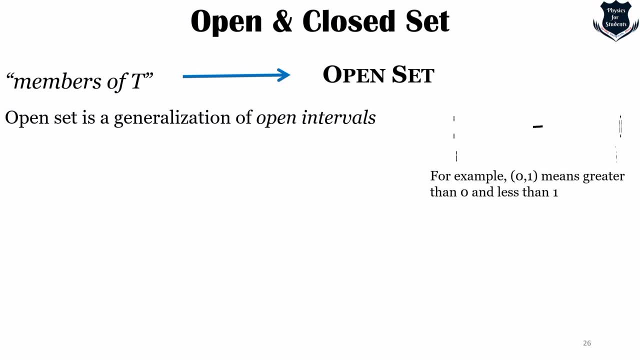 open intervals. We all know what is an open interval. for example, if you have 2 lines A and B and the lines do not join, we call 0 and 1 means greater than 0 and less than 1. so open interval, like the way it does not. 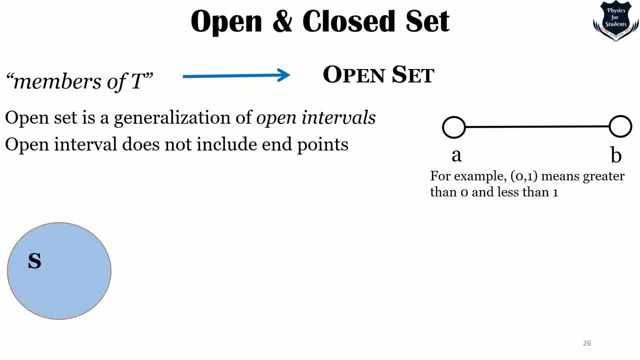 include any point. so does the open set. so now we take a set s and we take a subset t. now you see all this, this one, this one, these are subsets, right? so which has certain properties? again, definition, followed by important properties. so what are the properties? the first property is: 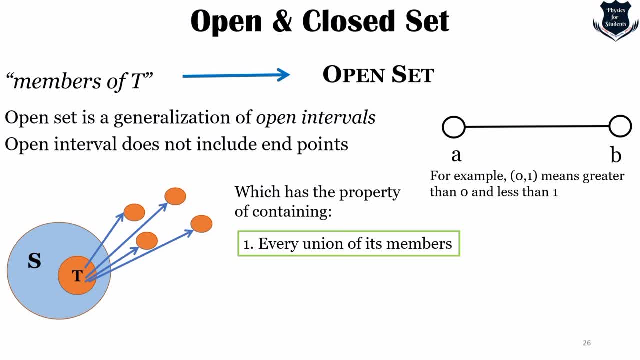 that every union of its members. now, what do i mean by that? it means that property containing every union of its members should be there. every finite intersection of its members should be there. there should be the empty set and the whole set itself, so a set in which such a collection is. 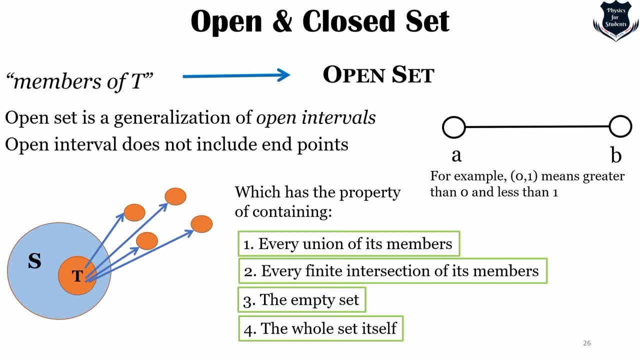 given is called a topological space and the collection is called topology. we have seen that these conditions are very loose and allow enormous flexibility, uh in in terms of choosing open sets. for example, every subset can be open right, or no set be open except the space itself and the empty set. so up till now we have understood that this is how we 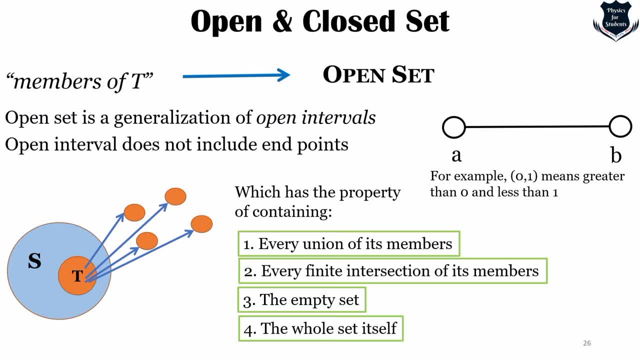 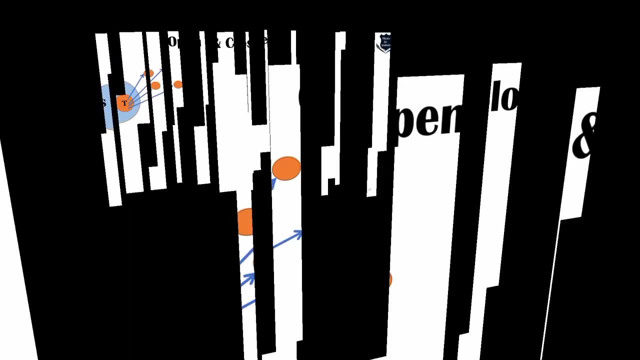 define an open set. it is just like an open interval. so open interval does not include end points. here also we are not including end points, and 1, 2, 3, 4, every union of its member, every finite intersection, the empty set and the whole set itself should be there. we will demonstrate further and things we will take on this example forward. 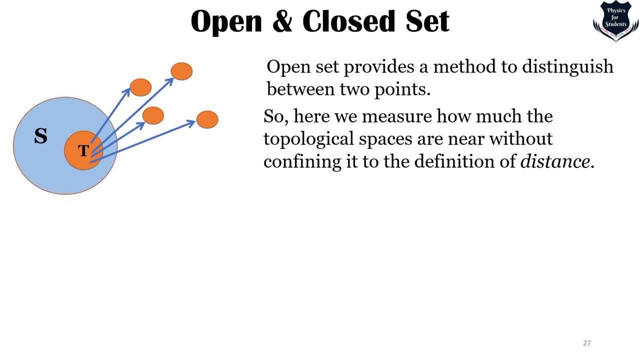 so open set provides a method to distinguish between two points. this is utmost important. so in order to distinguish between two points, see the next line says we measure how much the topological species appear without confining to the distance definition of a distance. so this is the subset. 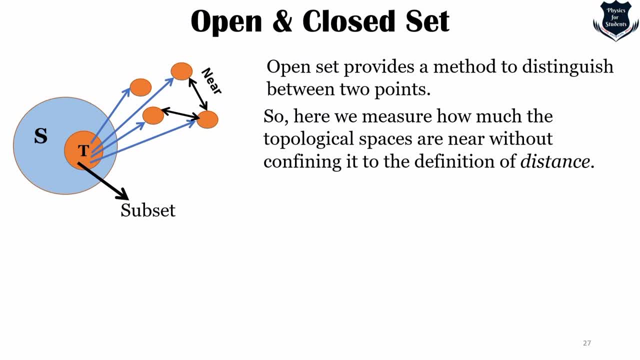 and these are the distances. distances means it shows how clear they are. ok, so this is very important. so the this with this by far becomes very important, because the the entire sense of topology has to capture the basic properties of closeness. so it turns out that there are two properties that 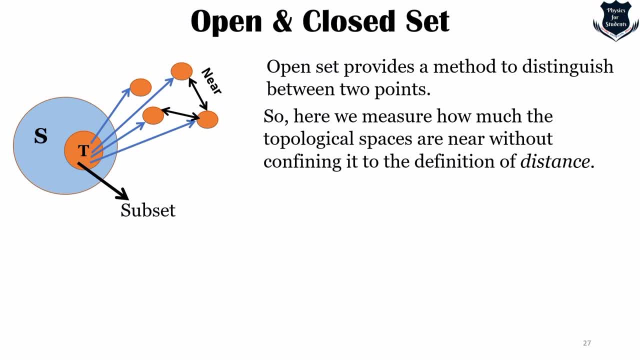 encapsulate the idea. we have just seen that these are that the union of any connection of open sets to be open and the intersection of open sets and narrative. so this will be the far most common. any two sets should be open. so what we are trying to do is that we are trying to measure the 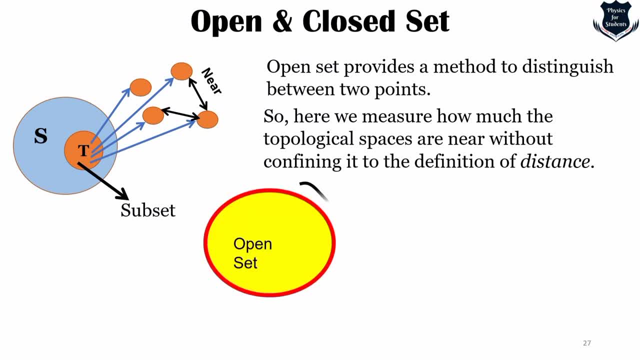 dearness. so here, the yellow set, this one, this, this, this border line, this is basically what is called it- satisfied this equation and the internal, which is the yellow one, satisfies this one, and what we do is that we call: the yellow set is an open set, the red set, the border is basically the. 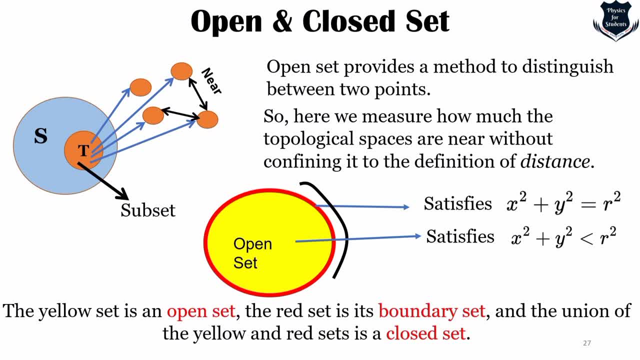 boundary set and the union of the yellow and red sets is the closed set which will be come later. so the you got the idea that open sets are basically providing a method to distinguish between two points. here in topology we don't call points, we call it members of the sets right, x, y or 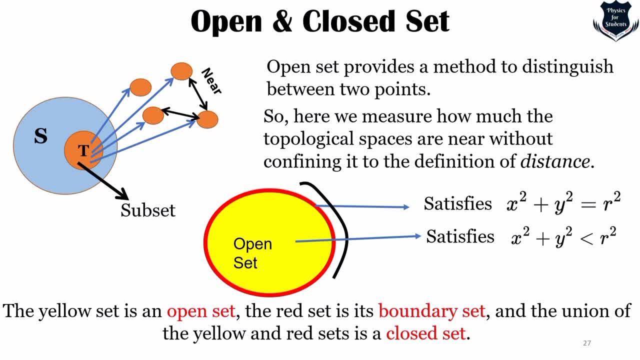 a, b, c, and we measure how much the topological spaces are near or far and do not confine it to the notion of distance. so the properties that encapsulate this idea and the the entire space is being defined using open set, so that the distance and the restriction 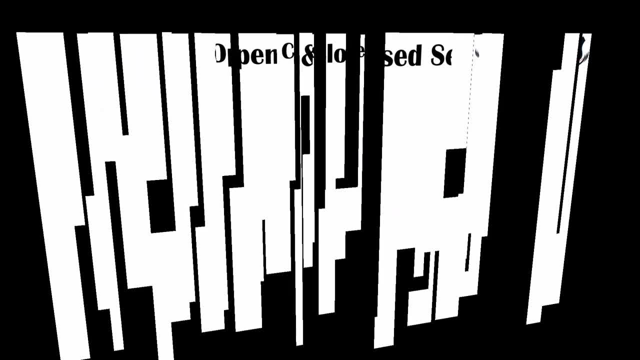 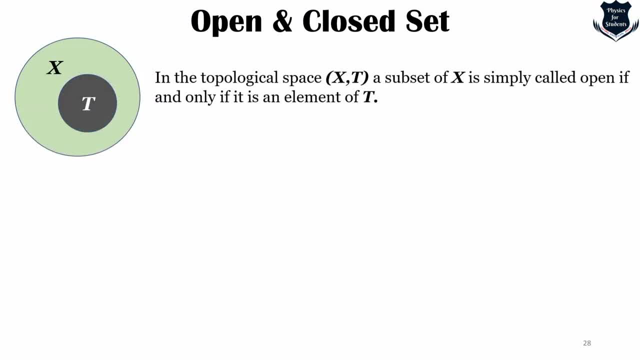 are not there, okay, so first we will see a further example, so if you go ahead with this one. so this is how we define the topological space x, t, a subset of x is simply called open if, and only if, it is an element of t. so rather than speaking of a concrete euclidean matrix, you one may use. 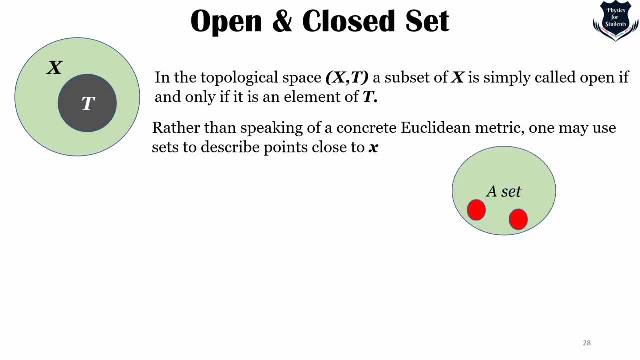 sets to describe points. for example, if this is a set and these are the points, okay, i mean to say we don't call it point and so this is, this is the one, these are the one, so these are other points should be sufficiently close to it. so the idea of open set is that for each point in the set- the red ones- the set should also contain: 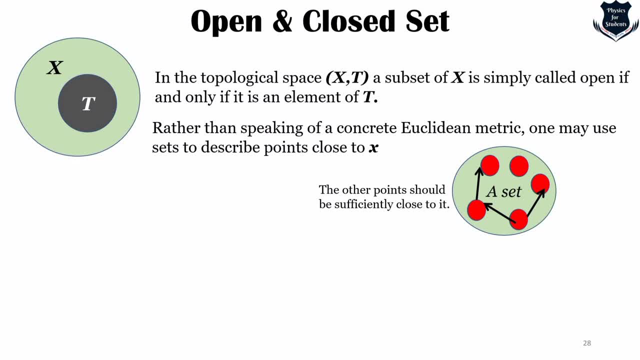 all other points that are sufficiently close to it. we can call it in a different way- that in you, we should be not be able to approach a point within an open set without entering the set. so openness is an. so in metric space we define by this and here we define by this. so openness is 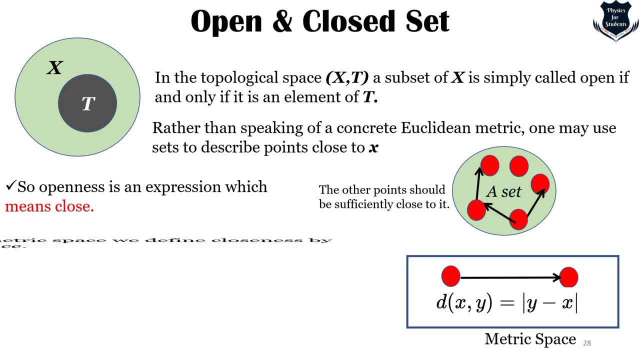 an expression of what it means to be open. so this is an expression of what it means to be open. so in metric space we define closeness by means of distance, but in more general setting, like topology, it is not possible. so instead we define closeness by a simple listing of what sets we want to be. 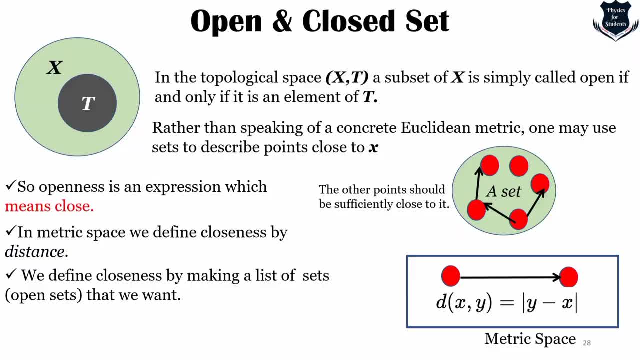 open, and the list is just a set containing all the open sets in the space, which is called the topology. i'm so sorry, wait, let me. let me quickly go back to this one. yeah, so this is how we define. it. is in metric space and this is how we define it in metric space, and this is how we define it in. 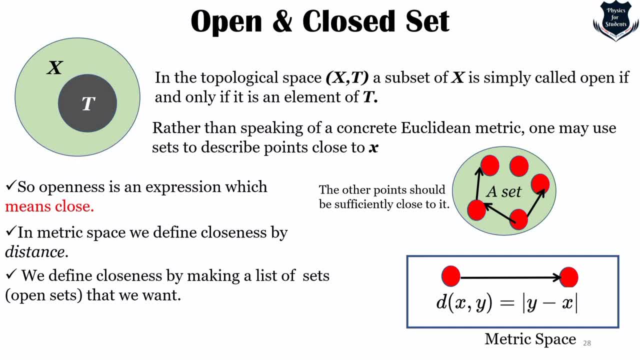 topology. so the idea again, i would repeat, is an open set, that each point in the set, the set should also contain all other points that are sufficiently close. as you see here in this right hand side, these red dots connect to the closeness right. so openness is an expression of what it means to be. 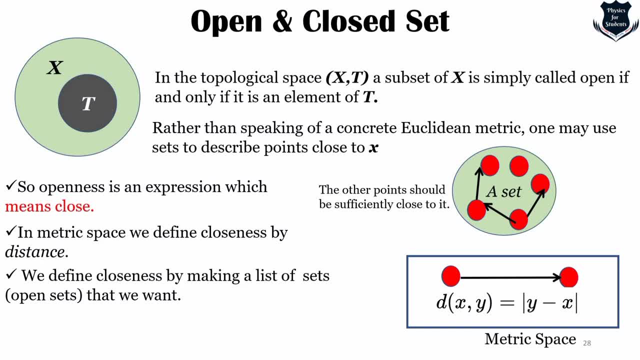 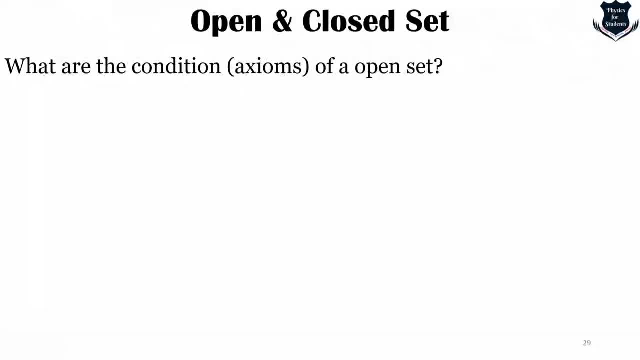 close. in metric space we define closeness by distance, but here we define by closeness. okay, where do we go in the next part of the video? okay, so what are the axioms? that means, as i told that, what are the conditions of an open set? first one is: the empty collection should be an open set. 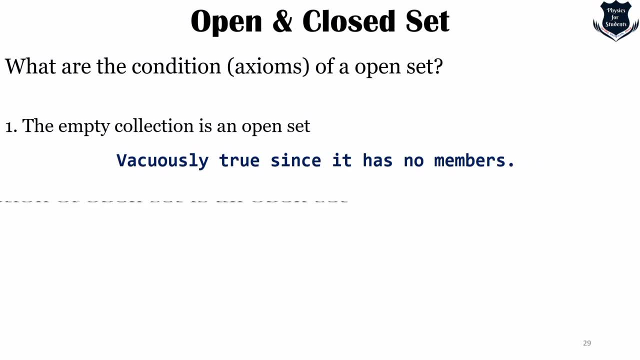 obviously, because this is true, since it has got no members. the second would be: an infinite intersection of open set is open. yes, because we just verify the membership in each of the open set all at one at a time, and the union of open set is open. so this is an open set and this is an open set. 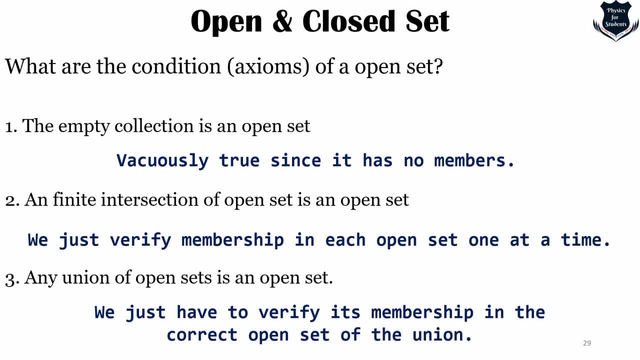 is an open set. why? because we just need to verify the membership in the correct option set, whether it has got an union or not. so these are the conditions which tells that, in order to become an open set, things will become more clear. okay, so we come to the mathematical definition of an. 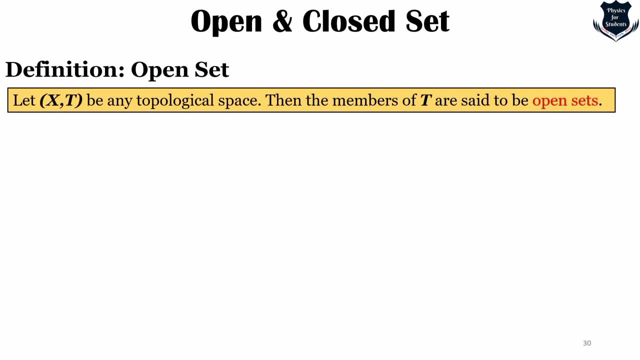 open set. so let x? t be any topological space, then the members of t are set to be open sets. if yeah, so we get a proposition from that. if x, t is in topological space, then the members of t are set to be open sets. if 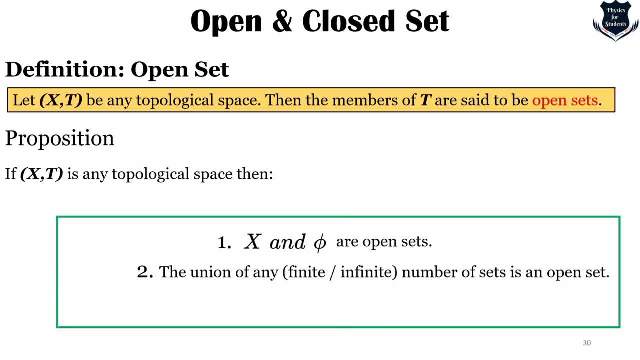 yeah, so we get a proposition from that. if x, t is in topological space, then x and phi are open sets. union of any finite or infinite number of open sets is an open set and the intersection of any finite number of open sets is also an open set. now it might crop up in your mind a question that here we are calling, on point number two, the union of any finite or infinite number, but various. in point number three we are calling only the finite number. so the question rises is that: 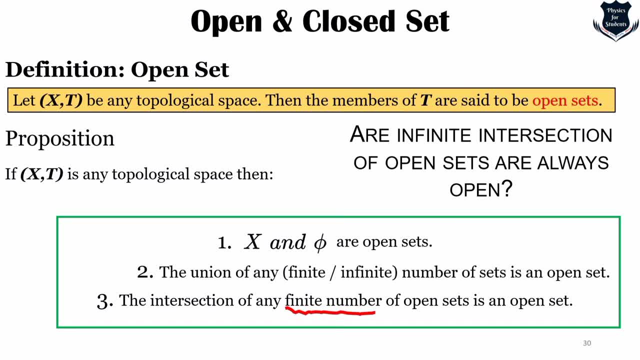 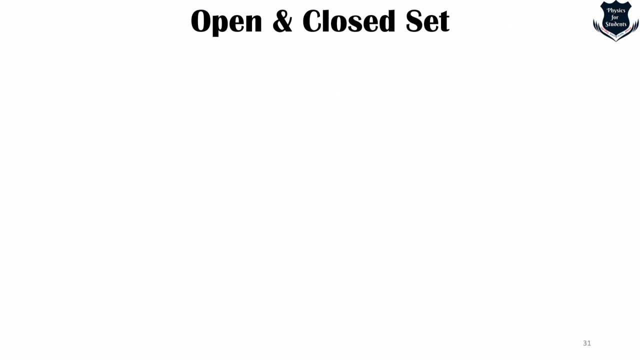 are infinite. intersection of open sets are always open because here we talked about finite, infinite, but here, when you're only talking of finite number. so if you get infinite intersection of open sets, do we find it to be open? let us find out right now in this video. so let us assume that n be the set of all positive integers, as we know, and let us assume that t consists of phi and. 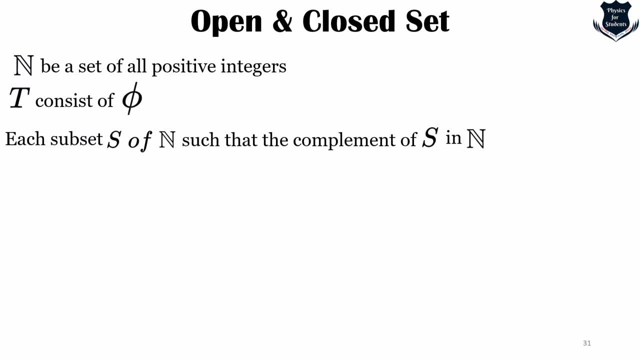 the, the complement, each subset s of n, such that the complement of s is in an and we do not it simply by this, which is quite known to all of us, and this is our finite set. okay, so we can easily verify that t actually satisfied this condition. which is satisfied this condition? the union. 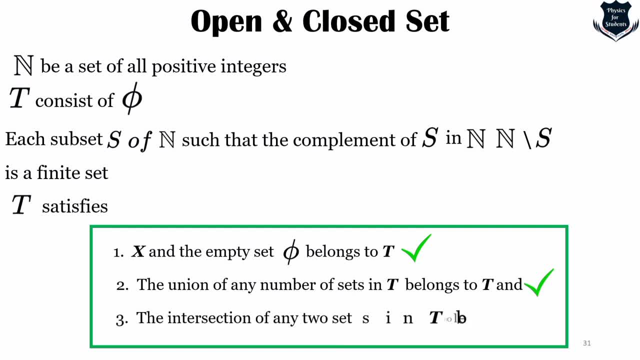 of number, this is also satisfied. and this number, the third condition, it is also satisfied. so we can tell terus, T is a topology on n. So right up till now this is quite simple. What we are trying to find out is that whether that can be called as infinite topology. 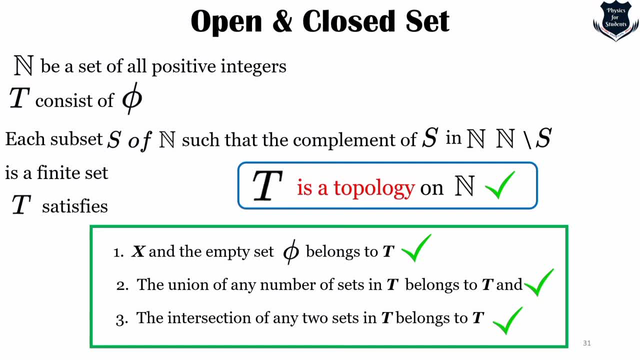 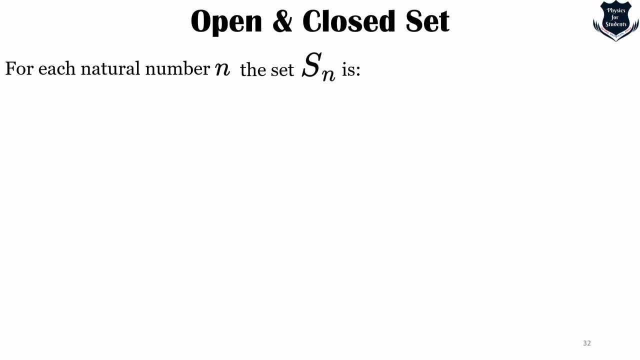 infinite space is called. So T is a topology. on n. Now we have find Now if. now what we do is that if we assign a natural number, n, so that the set S of n is something like this, So what we have done, I have just added: 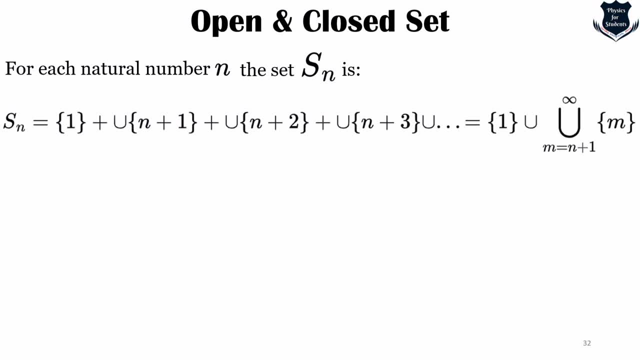 union of n plus 1, n plus 2, dot, dot, dot, dot, dot, and it goes up to n plus 1, up to infinity. Now, obviously, from here, what is very clear is that S of n is an topology on n- right, It is an open set- and topology on n, since its complement is finite set. 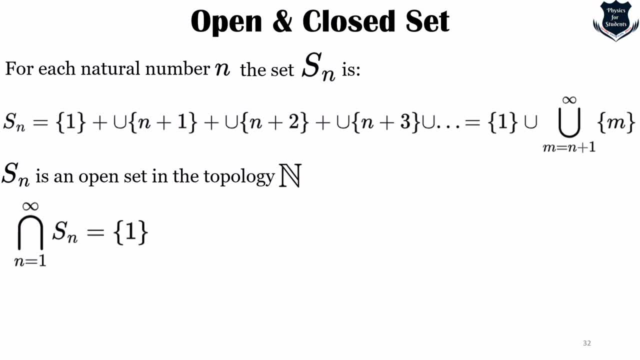 right So, but when we take this kind of a thing, right, yes, when we take this kind of a thing- then what we see? that the complement of 1 is neither in this natural number, n or a finite set. 1 is also not open, So 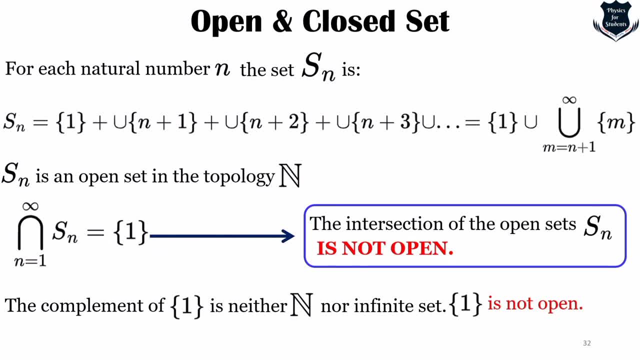 what it proves is that this part of the equation says that intersection of the open set S n is not open Now. so so we have proved that this one is not open. So we cannot call that infinite number of intersection of open set can be open. We. 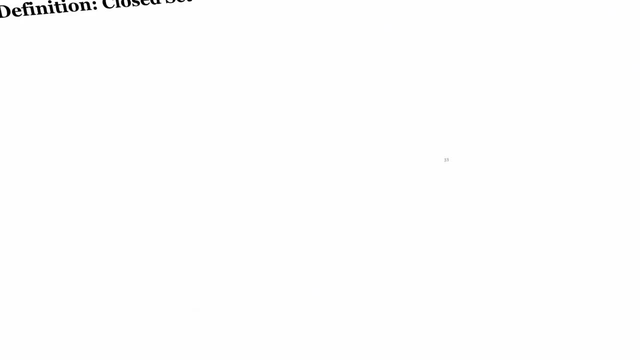 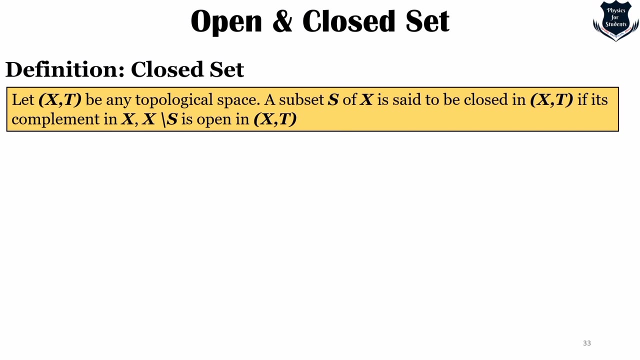 have just proved this. Okay, so where do we go from now? We now we define what is a closed set. Very simple. Let X of t be any topological space, then under subset S of X is simply closed if its complement is open. This is just the reverse. So we call it. 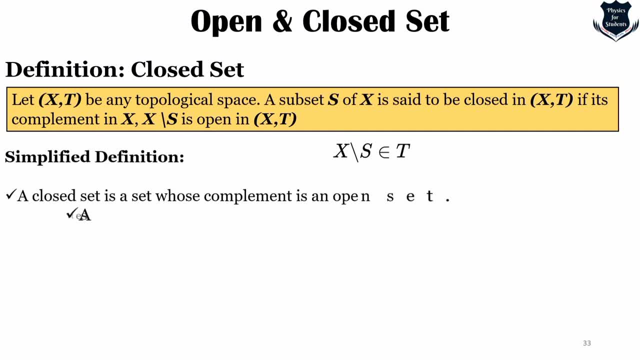 like this, and if I want to make a simplified definition, it will be something like: a closed set is a set whose complement is an open set, and it has got only at its limits: forms. Now, if we take the very first example, when we were defining topology and 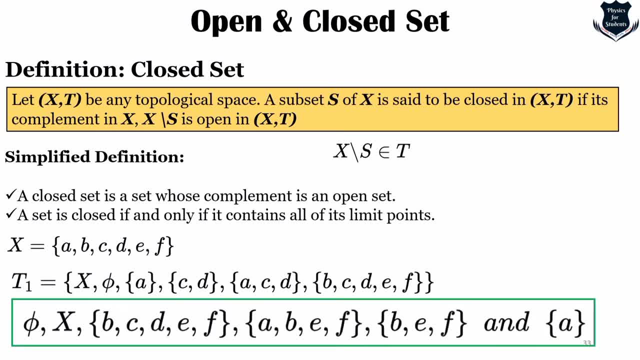 topological space, then if you rearrange them in this way, then we find this to be a closed set. I am not going to explain it right now. I would say how this is going to be an open set is just that you see the complements then X, P, C, D, F and. 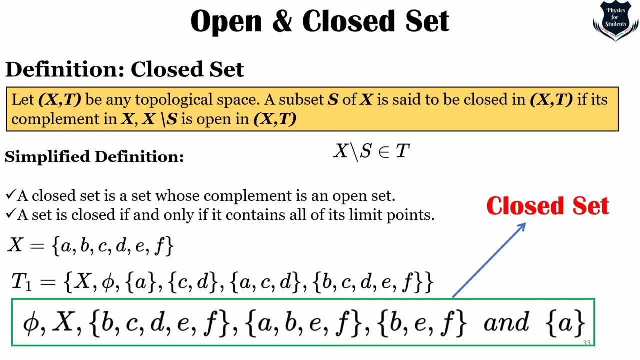 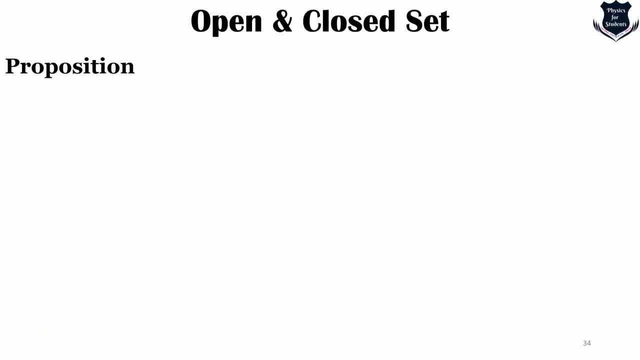 you arrange, then this becomes a closed set. This is just to give you an example that how we can use these points or these elements in order to define a closed set. Okay, so the proposition from it comes is that if X, T vary any topological space, then first phi and X are closed sets. the intersection of 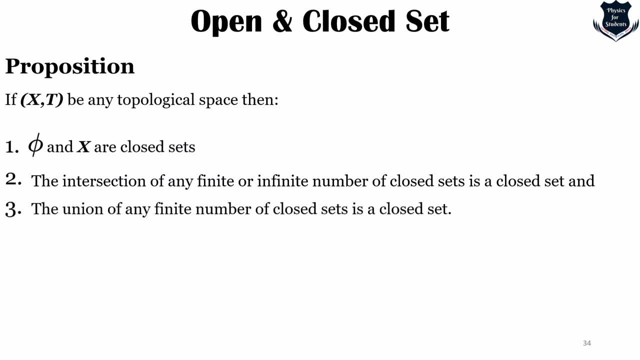 any finite or infinite number set is a closed set and the uniform union of any finite or infinite is also a closed set. So the first part, phi and X, are closed sets. how we can prove It is simple, because X and the empty set, phi, belongs to T, so phi and X are closed. 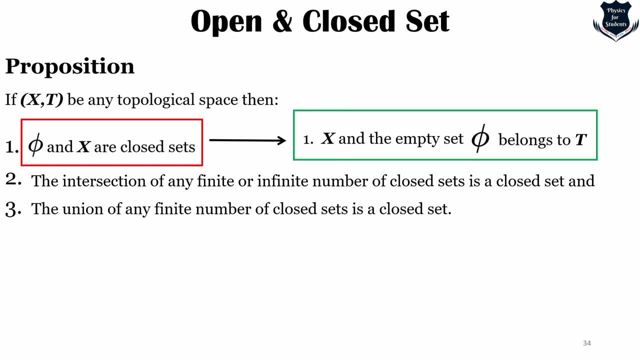 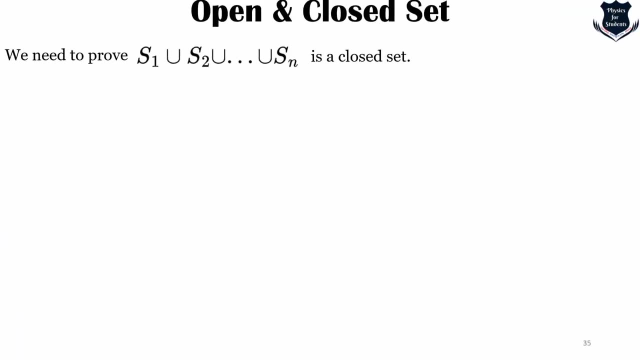 set. that comes from the rules of the. you know this complementary part, So this is being proved. Now what we need to prove is the second part, that S1 union, S2, dot, dot, dot, so on, is a closed set. So let us see how we can do that. So we need to prove this, this. 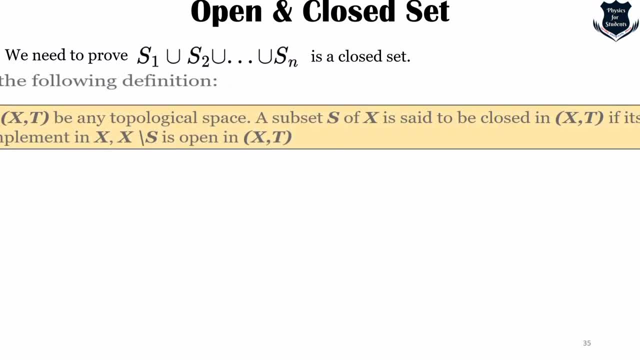 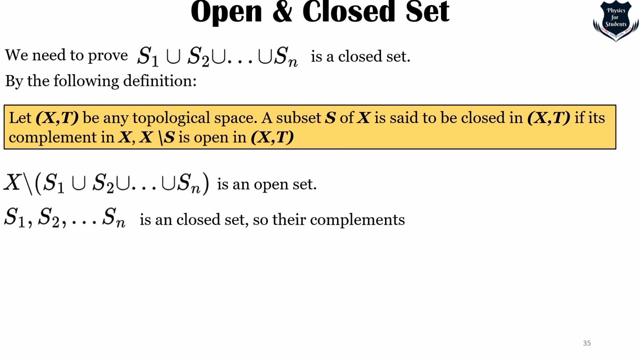 is being known. Now we are required to you know. if we take this definition, which is the definition, this one, let X, T and the closed set, then what we see here is that this one is an open set. Why it is an open set? Because S1, S2, dot, dot up to Sn is a closed. 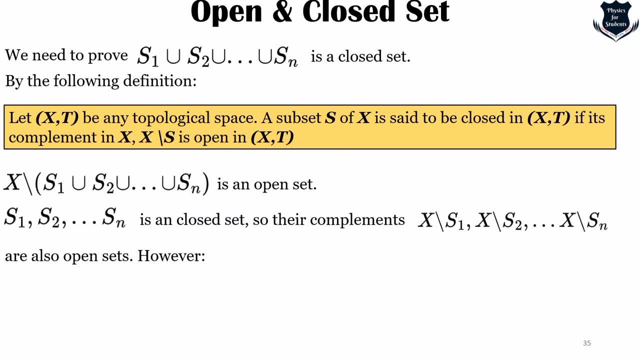 set. so their complements, this one are also open sets. But however you see this, this one, If I form this in the union and the intersection of X, then this left-hand side part- sorry the left, yeah, the left-hand side part- is an open set because it is a finite collection. 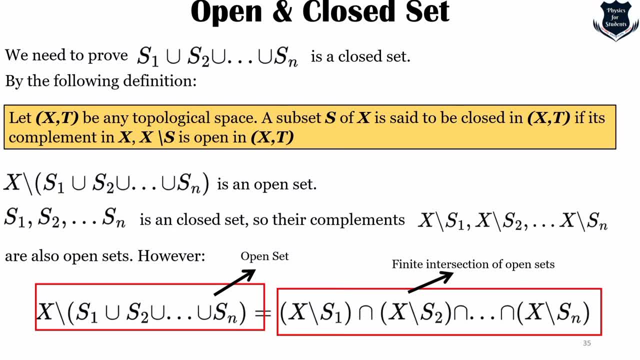 and this is also a closed set. So this one is an open set. So this one is an open set. So finite intersection of open sets. So from here what we can deduce is that, yes, S1, S2, dot, dot, dot, Sn is a closed set, So the right-hand side is a finite intersection of. 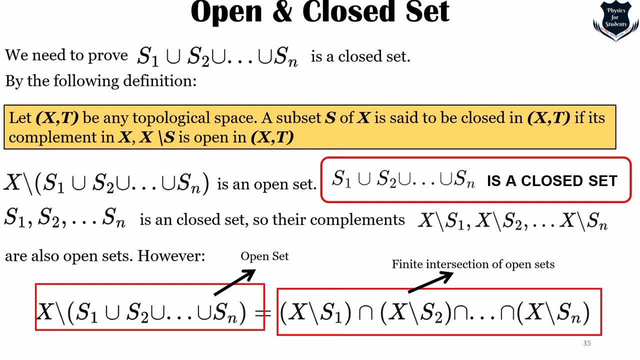 open sets. So, and if it is open set, the left-hand side of the is also is an open set. So from that we deduce that S1, S2 and Sn is an open set. So that is how we define. 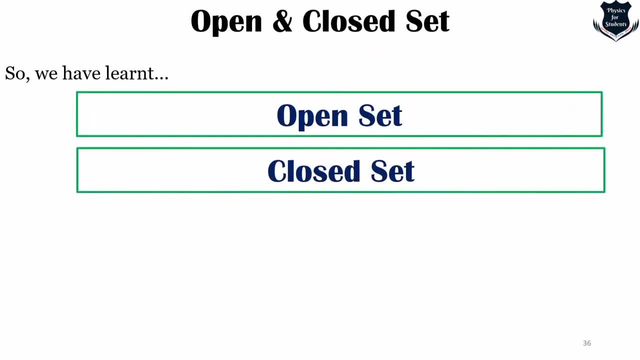 what is an open set, and we do the different theorems and calculations. So up till now, what we have learnt is that there is an open set, there is a closed set, But what about both Then? can we have something which is both open and closed? 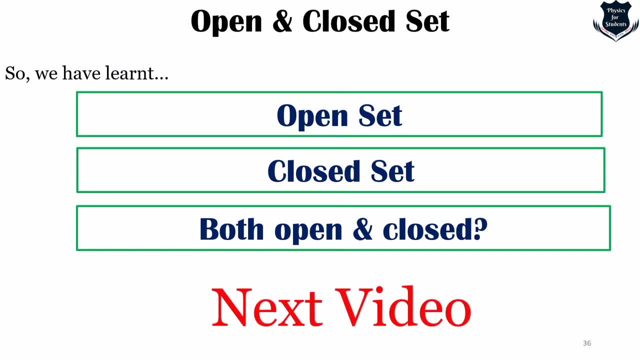 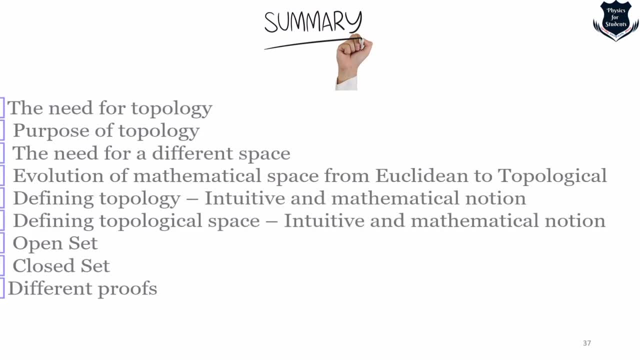 Yes, the answer is yes, and that will be the next video in which we will be learning that. So we have come to the end of this video. Let us summarize what we have learnt. We have learnt why there is a need for topology. 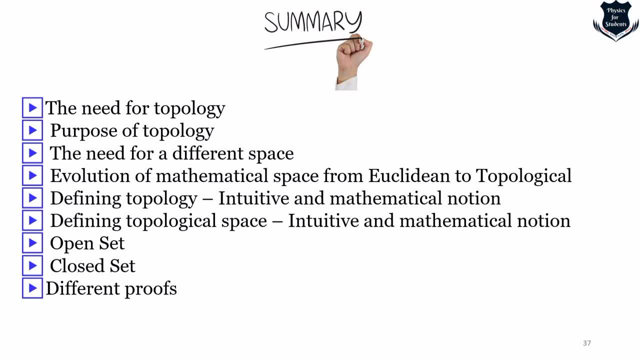 What is the purpose of topology? There is a need for different space because Euclidian axioms won't work. So the evolution of Mathematical space from Euclidian to Topology, Defining topology intuitive and the mathematical notion. We have also seen what is the topological space in terms of illustrations and mathematical 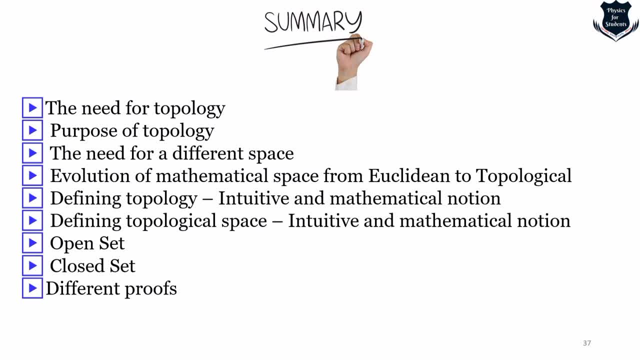 notion. We have also seen what is an open set, a closed set, and simple proofs which would prove either it is an open set or closed set, or a closed set or union or something like that. so this completes our video today. if you have missed my other video, i would request you to look into my playlist, because that video was the. 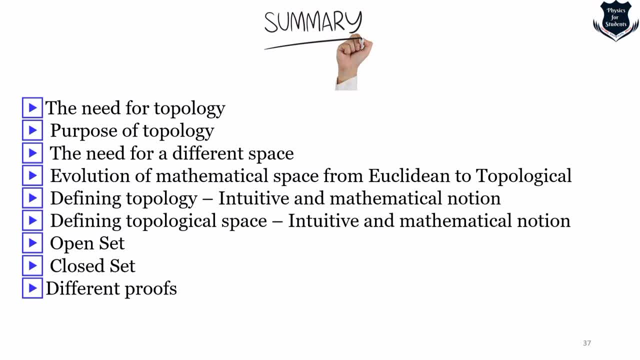 foundation. so we are dealing with those fundamental concepts one by one. so in the next video we will see what is both open and closed set and further, what are the concepts like compactness, closeness, etc. which will be coming up in the next video. thank you very much for watching this video. 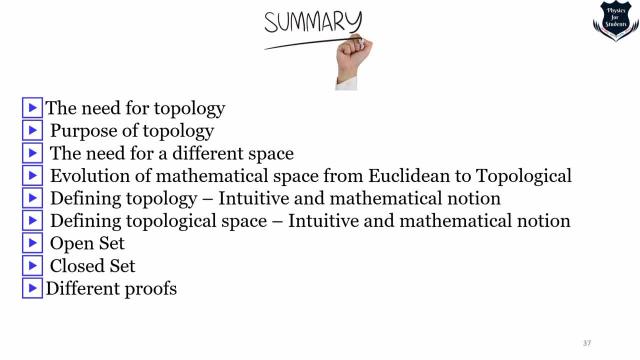 you have been a tremendous support, so please keep on supporting me so that i can keep on producing more and more videos of physics and mathematics. please do click on the bell icon and click on the all options so that you get all the notification about videos and interesting topics from physics. 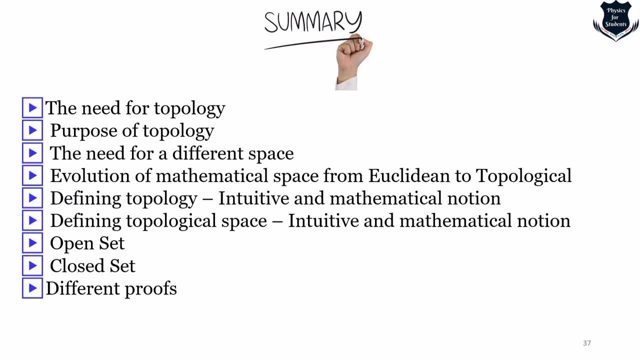 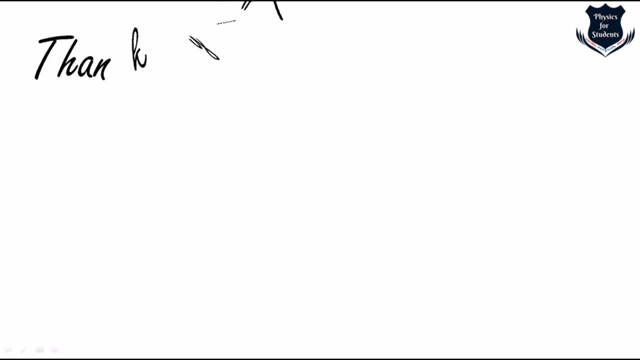 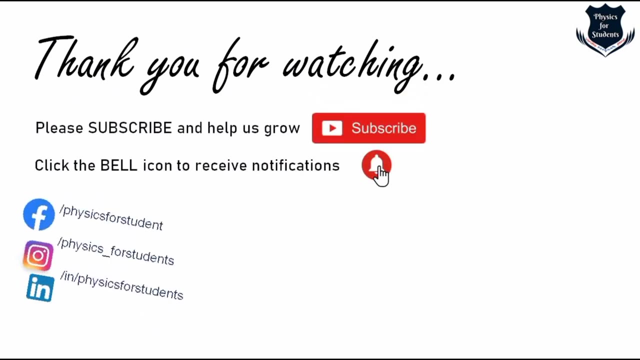 for students. this is shaunak signing off today from physics, from students, wishing you a great weekend ahead and promising you to come back with a very interesting topic on physics and mathematics. till then, all the best, best wishes and goodbye. now you can be a part of our team. you can send your scientific articles. 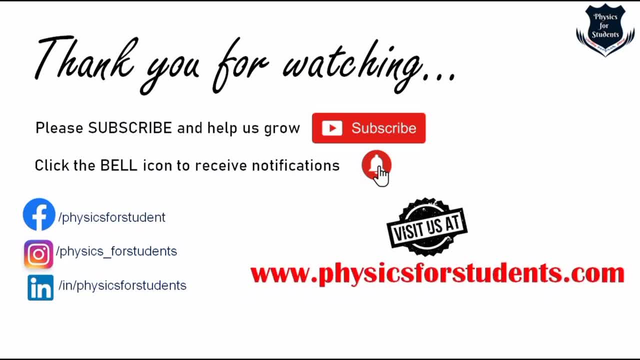 essays, research papers, lesson plans on a particular subject of science. for further details, please write to us at editor, at physics for students dot com. stay safe and happy.